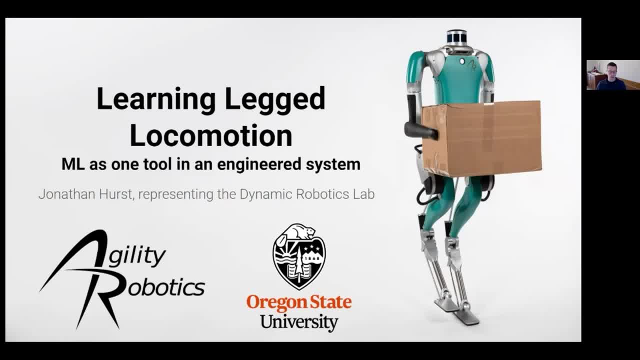 As Sam said, I was a mechanical engineering- you know- undergraduate and my whole kind of skill set. my talent is in designing machines But also understanding dynamics, And so I work with some really really great people in terms of Writing code and doing the software that controls really well. And what we're trying to do is kind of merge those things, Merge our understanding of how does legged locomotion work with. 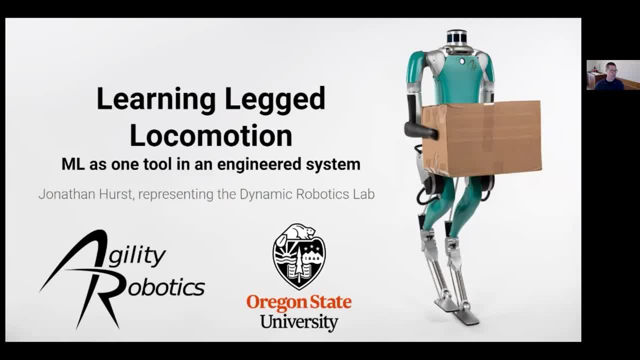 Some of these newer tools like machine learning, but it's just one of many tools And I don't think that you ever want to use it as a Kind of a black box solval. You just want to use it just along with all the other tools for engineering control systems. So that's what I'll talk about today. 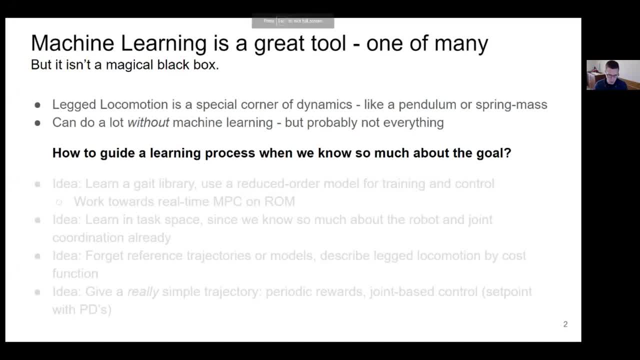 Okay, I guess I said this already, but machine learning is a great tool. It's one of many. It's not a magical box, And what I'm going to talk about for the first bit here is How legged locomotion is basically a special corner of dynamics. It's kind of a dynamical phenomenon. It's like a, like a pendulum, and the way the pendulum keeps time, or a spring mass system. Same thing, It's periodic. 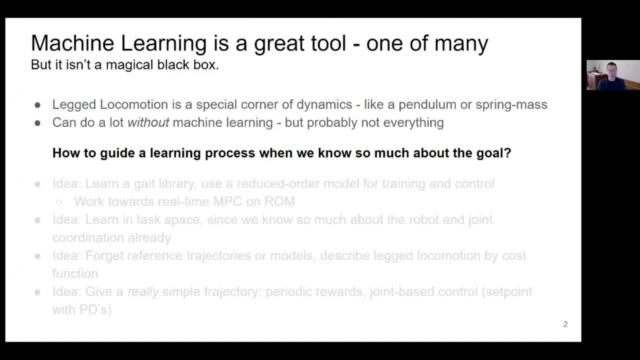 And- and I think something, something like that is the foundation of legged locomotion. It's not just Dynamics in general- try to get robots to do arbitrary things- It's more: capture this special corner of dynamics and work with it. And there's a lot you can do without machine learning. most of legged locomotion progress today is is without machine learning, but I don't think you can do everything. I think too much of. 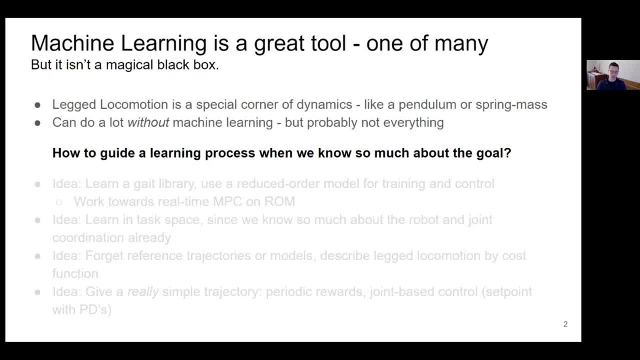 The approaches to date are our model based. and models are. what do they say? all models are wrong, or but some are useful. Certainly, models are always simplified And the question is, how do you do that? How much simplified? you know it's a reduced order model, but how simple is it not capturing all the dynamics of the robot? 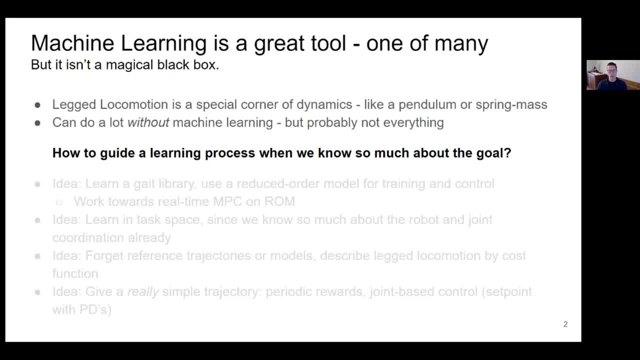 And if you really want to get into the corners and really get into all the dynamics that a machine can achieve, I think that that's going to have to be done with strange nonlinear representations that that can probably be learned with machine learning. So the question, though, really is how do you guide this learning process when we already know so much about the goal? 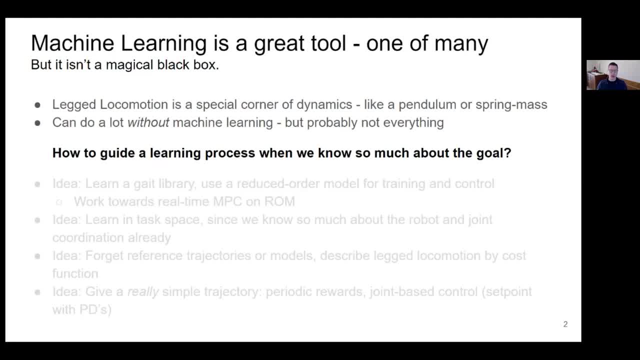 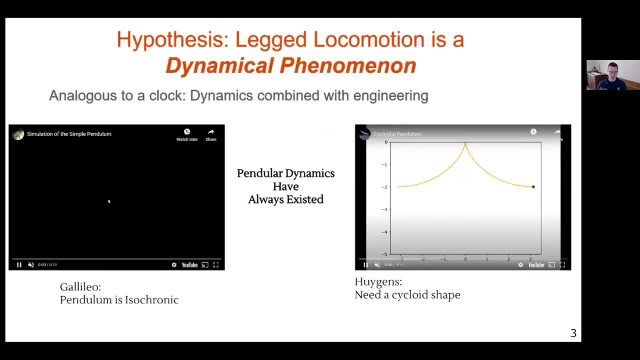 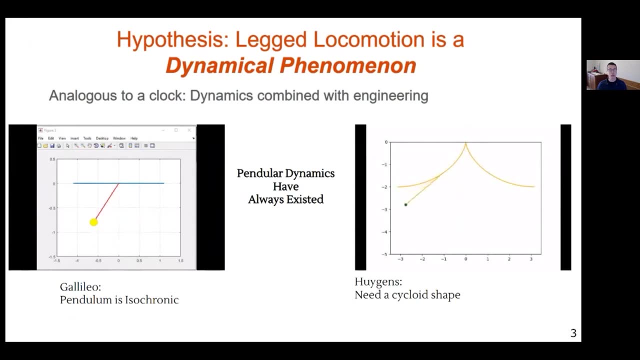 There's a lot of science We know about legged locomotion, So how do we then incorporate that in steer our learning process, given what we know? Okay, So to start with, here's the hypothesis right: legged locomotion is a dynamical phenomenon. It is in many ways analogous to a clock. 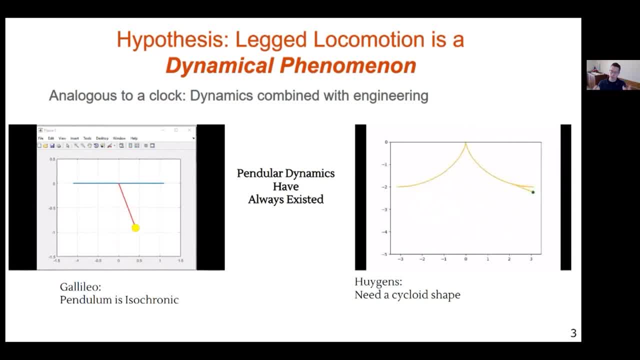 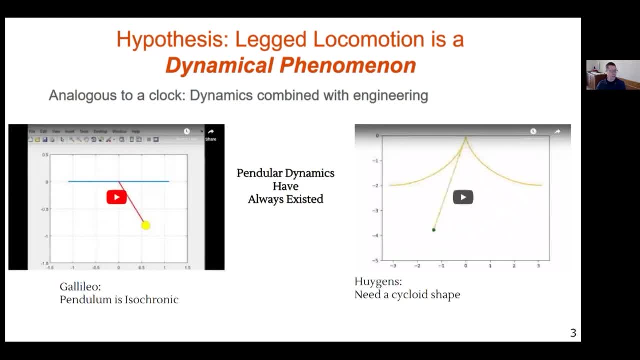 And I would call that. what I mean is it's dynamics that exist. These are just physics that exist, combined with engineering. Now, early on, Galileo just made the observation: Hey, if I swing a weight scale From a string, it's isochronic, it keeps time. no matter what the amplitude is, the frequency stays the same, and that's a really interesting observation. just a physics. 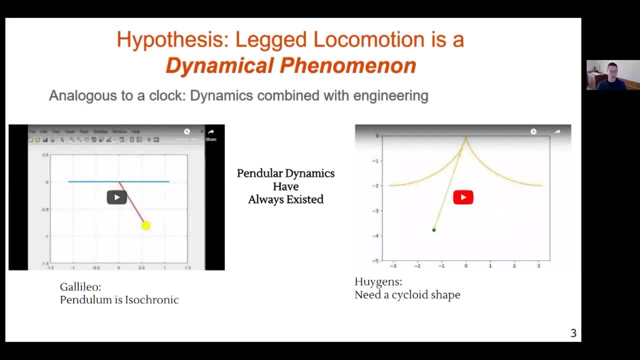 But it was not until, I don't know, 100 years later that Huygens actually did the math and say: actually you need a cycloid shape and afford in order for it to be actually isochronic. you know, here's the actual solution, Here's the 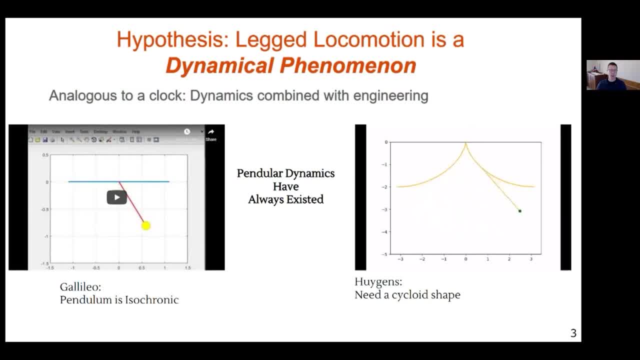 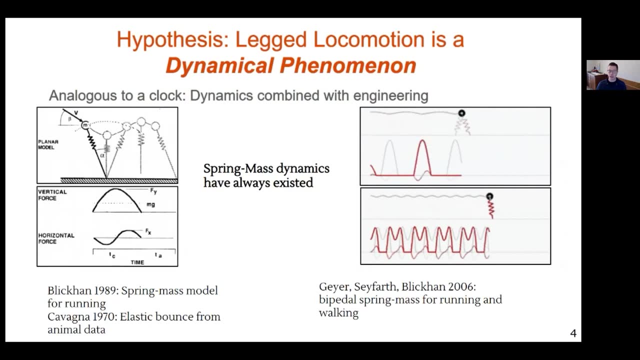 Absolute, you know, correct, perfect solution. And I think where we are today is More in the Galileo side, where we've kind of made some observations that you know, this spring mass behavior Really gives us some stability. And here's a simple model. This is very much a reduced order model but it describes some really interesting things that we observed in all animal locomotion. 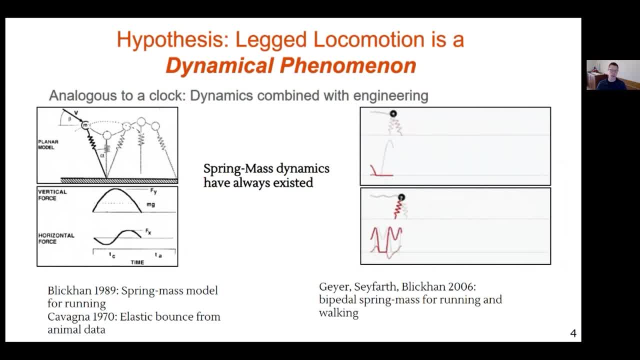 It's very, very self stable. It's very robust. There's a lot about this that is really interesting, that we think is kind of a Just a. this is a special corner dynamics. This is sort of like a discovery. But again, I think this is kind of the Galileo version of the pendulum, where maybe this is capturing 80% or 75% correctly. What's really going on? 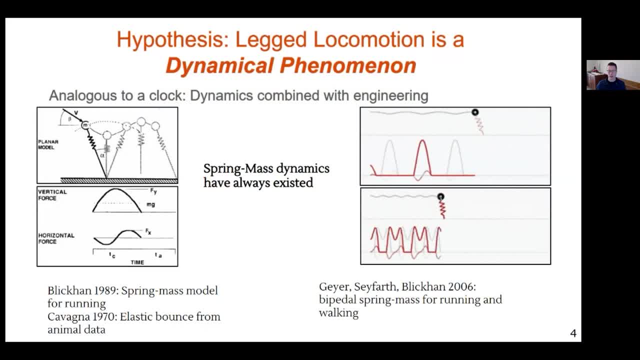 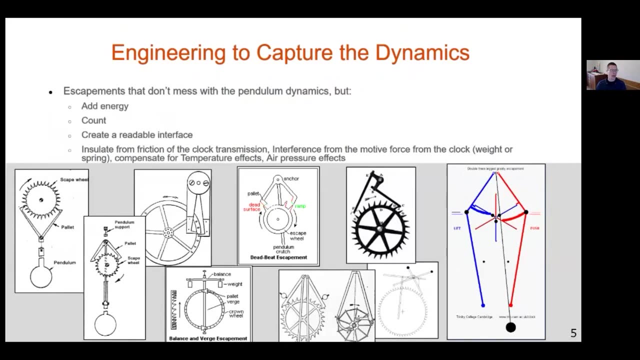 And we have yet to understand really what is the full, perfect picture of this dynamical phenomenon or how to utilize it. That's okay, Still still useful. And then I talked about engineering to capture the dynamics. If you think about A clock, 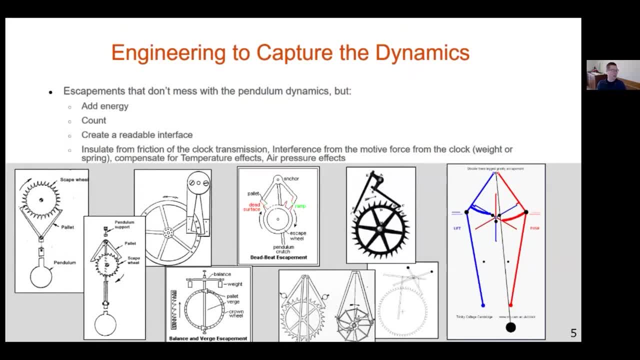 It's not just the pendulum. you know you have to add energy to it, You have to count up the number of swings, you have to create a readable interface, You have to figure out how to insulate your pendulum from all the friction and all of the interference and all of the 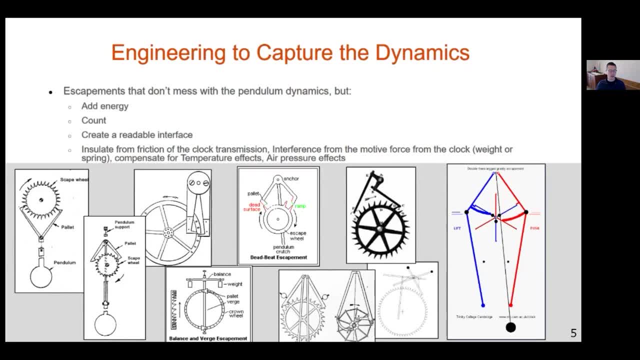 Dynamics of your gears and things like that, or the weight or the temperature effects, air pressure or all the other things in the clock. So hundreds of years of engineering went into making clocks decent time Keepers, With the pendulum anyway, and you know, eventually of course they went to quartz crystals, which are oscillators and electronics and in and so on. But let's ignore all that for now. Let's talk about the special corner of dynamics. It is a pendulum. 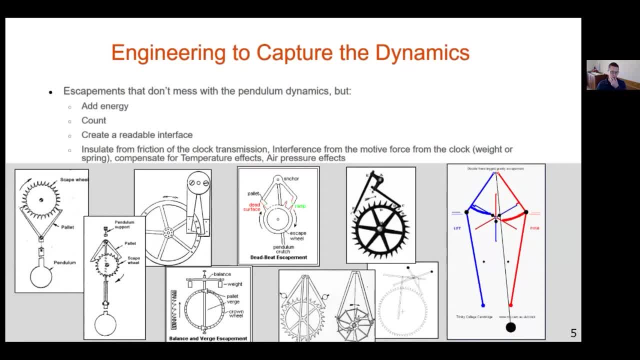 And how, the analogy between that and legged locomotion. By the way, I welcome anybody to To speak up and ask me a question. All right, I think I've left plenty of time in the presentation for questions, So just let me know. 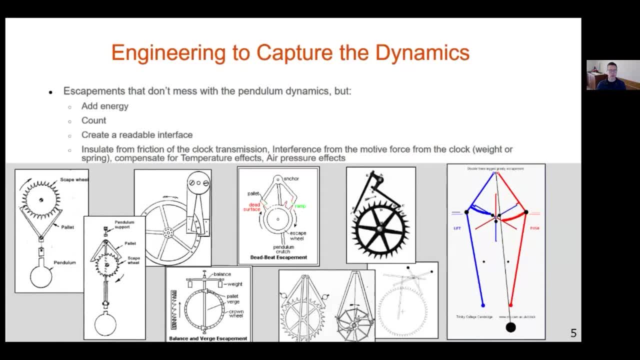 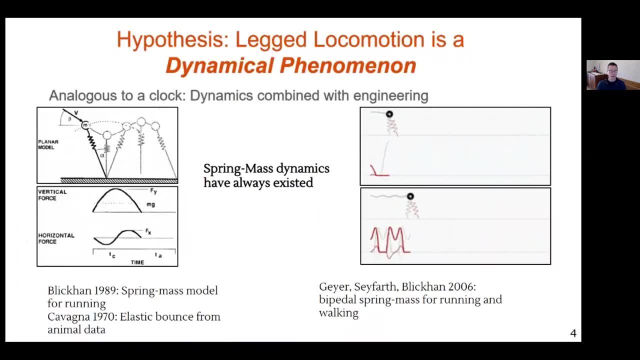 Yeah, I apologize, I forgot to mention those logistics and I'm monitoring. you know the participant window in the chat, So folks have questions, they can type them in there, raise their hand or things like that. Great, Okay. so legged locomotion is a dynamical phenomenon, something like a clock, but there's a ton of engineering you need to do. 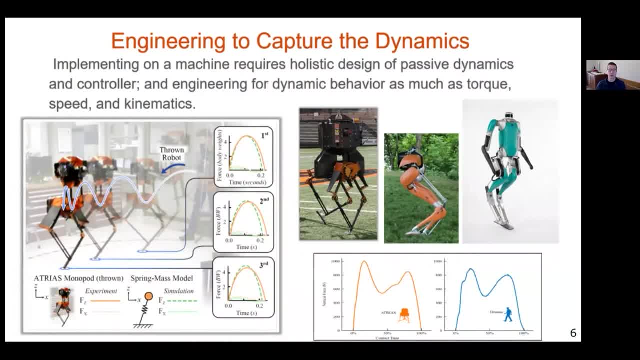 And here's some of the engineering to capture the dynamics for legged locomotion. now, early on, what we did is we said, Okay, I think we understand that this spring mass model is is at least close. right, it's something We're, it's, it's. it's not just a descriptive pattern, It is very close to what the actual physics are that give us stable behaviors and robust behaviors and efficient behaviors. 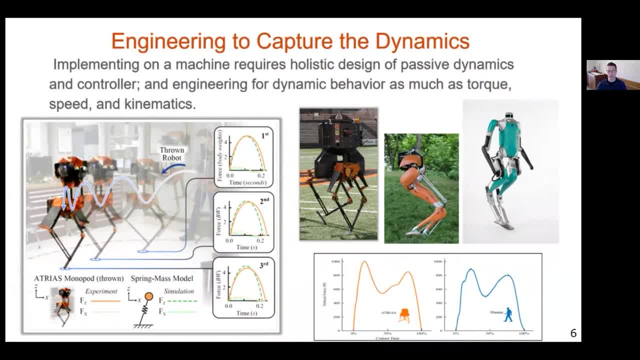 On animals and then you know should be able to do on machine. So we designed atrius, which is an acronym for: assume the robot is a sphere. The whole idea is to build a robot, build a machine that is as close as possible to the simple math model and early experiments. here you can see the 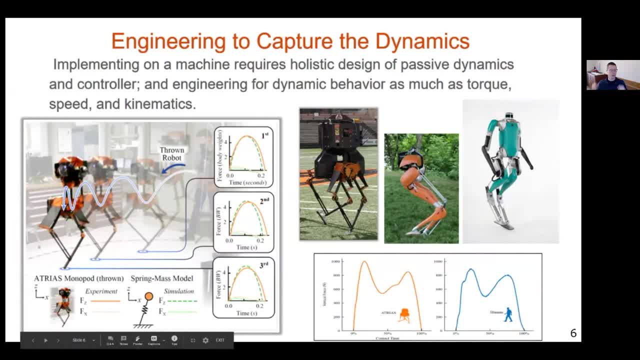 Force and the ground reaction force. when we pick up the robot and throw it in the air, the motors are turned off. It's just going to bounce a few times and we're getting pretty close to the ideal spring mass model. The green dash line is the simulation. The orange line is what the robot actually did when it landed on the ground. 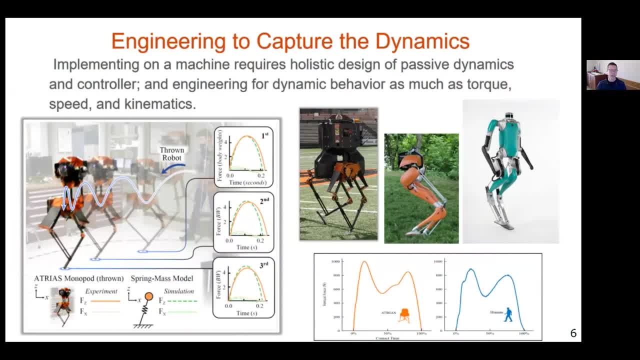 So we built something really close to a spring mass model. Okay, then we built it into the full bipedal robot and we were able to get atrius to Do continuous transitions through the speeds between walking and running, which reproduced exactly what we saw in simulation. We're very early on in the program. We were able to walk and run over all kinds of terrain. 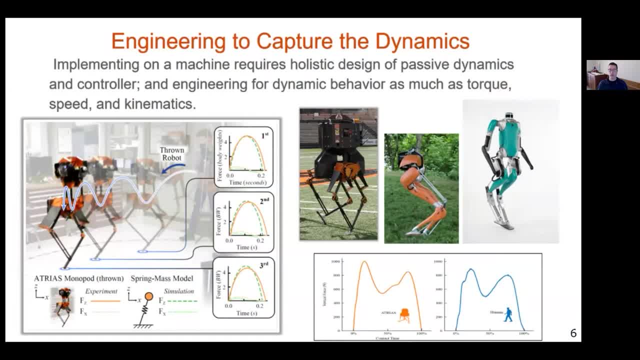 Unexpected step ups and steps down that were significant fraction of the leg length. It didn't matter what surface we were running on, so grass or pavement or soft foam, It just it was self stable, just shrugged off all of those sorts of things as a dynamic behavior, And so this was a really important demonstration of the idea that 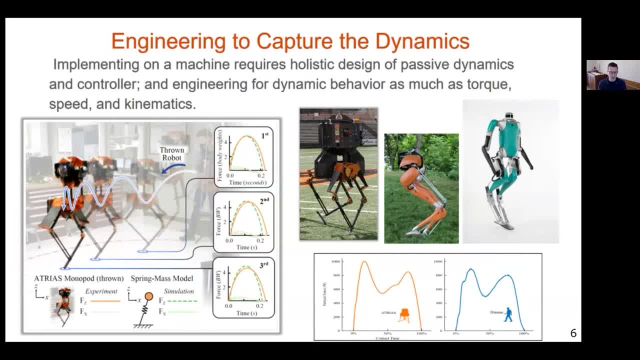 We, we are in a special corner of dynamics. It's only dynamics that is causing this robustness. There's no planning, There's no perception, There's no decision making. It's just a spring mass system with a very simple controllers on where it's going to place the feet in order to stay balanced. 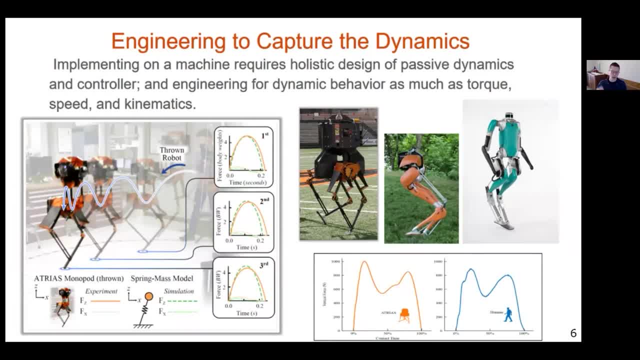 And then there were a bunch of other things that that were pretty important about what happens at impact and what is your behavior going to be through that impact, And that's why there's giant physical springs on atrius. So you know you could do it through actuators, if your actuators are good enough, but you still want your behavior to be a certain thing. You still want your 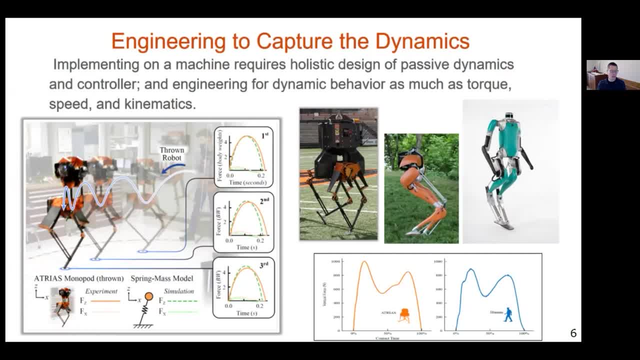 The dynamics that you engineer. However you engineer it, you engineer some behavior through your actuation and your passive dynamics, to be something when it's going to encounter or impact the ground. It's a holistic design And so you can see here the the ground reaction forces of atrius running over the force plate. 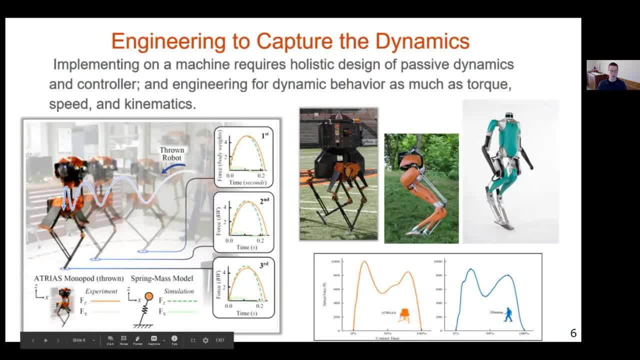 And compared to my graduate school At the time, Christian- who big he is now a professor- Running across the force plate, You don't see a huge difference. at least the high level structure of what you want to see is there. So that's, that's good evidence, that is on the right track. Okay, so that was a good science demonstrator. atrius was: 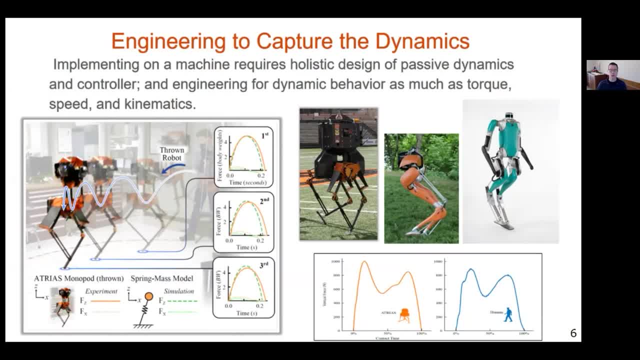 We then started going towards robots that a little bit more useful with the Cassie robot which, which we sold to some of the top universities through agility robotics, And now with digits. So we're still capturing the same physics that we understood from atrius, but adding quite a lot of perception: arms that you can balance when you're walking and and other things. 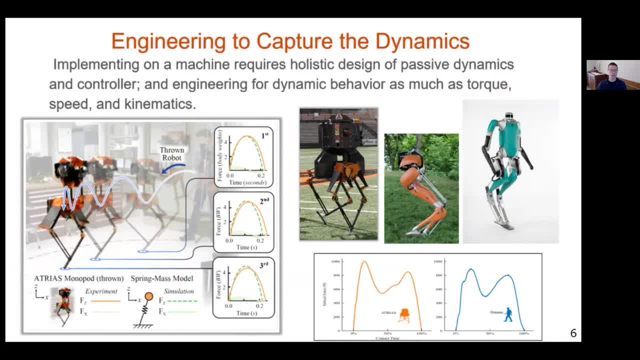 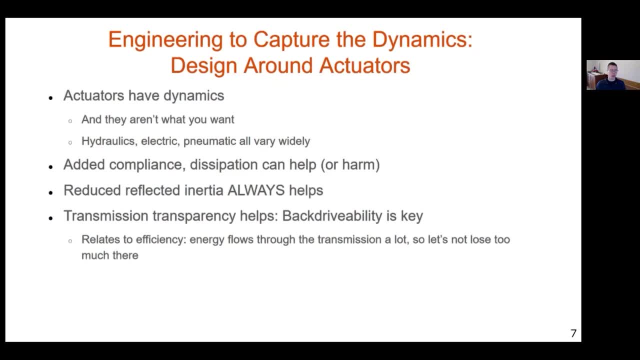 Capture the same physics but let's you do a lot more with it, like you want from a real robot. So I talked just a little bit about the actuators, And I think this is an important point. actuators have dynamics. They are a physical thing and they are definitely not what you want them to be. so a lot of the machine learning demonstrations and simulation or control demonstrations for like a locomotion have been with 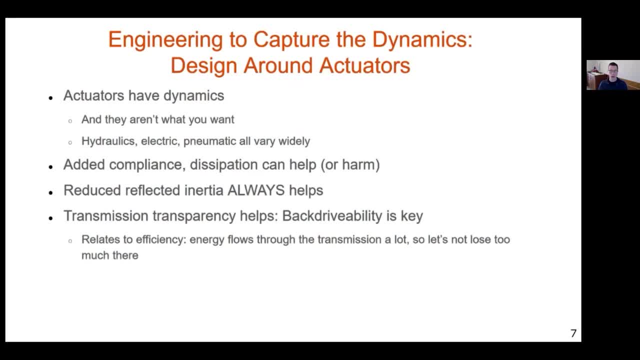 You know simulated robots where you can apply the torque that you wanted, every joint, and that will never happen on an actual, real robot. In addition, the actuators, especially the ones we use, the electric actuators, Have a lot Of what we call reflected inertia. 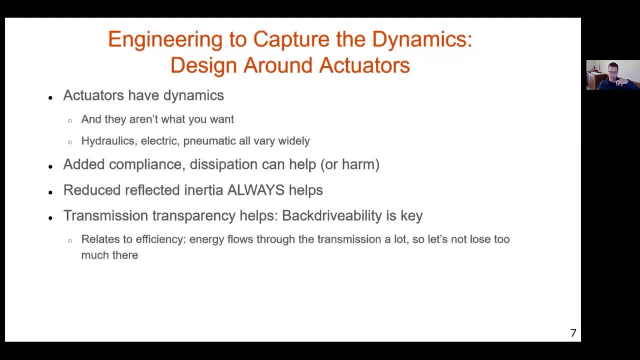 And so that just means there's a huge. you know the when you instantaneously change the speed of the output by a small amount, the motor itself, the rotor, has to change the speed by a very large amount because there's a gear ratio on it. 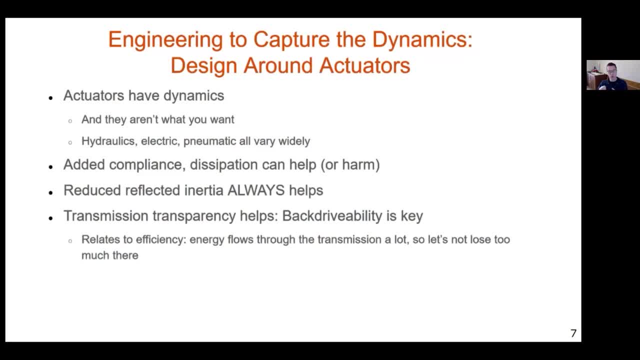 And that reflected inertia of the rotor spinning up that you feel through. the output can be very, very large, can be on the same scale as, as like the mass of the entire robot. So when you take a robot that maybe has 101 gear ratio. 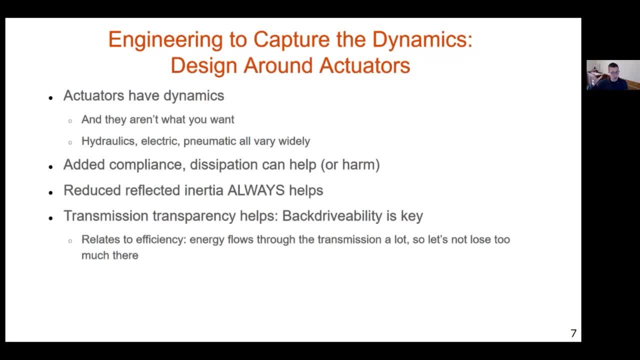 So when you take a robot that maybe has 101 gear ratio, Like a harmonic drive at the knee, and you were to lift it up and drop it on the ground, you're basically causing an inelastic collision between the reflected inertia of your motor and the mass of the robot, and it doesn't matter what software you write. 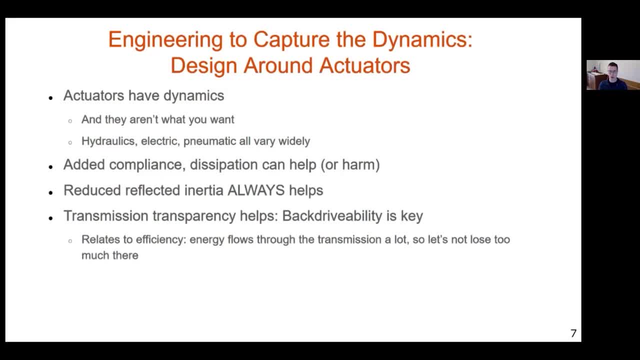 It's going to be that way because it is physics and it just exists in the hardware. So really, what you've got to do is deal with that. You can add compliance, you can add dissipation, you can add passive dynamics. Those things can help or harm. 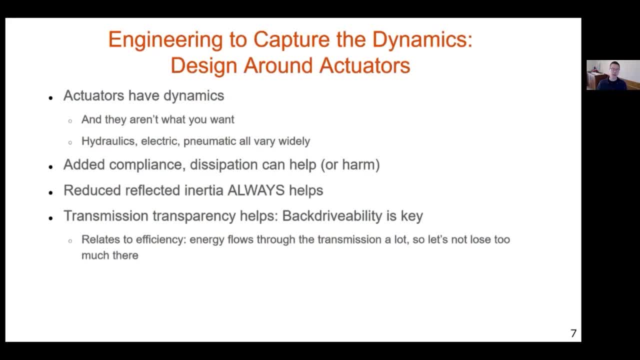 But you know, if you can eliminate as much of the actuator dynamics as possible, that always helps. So when you see like the Boston Dynamics Atlas doing backflips, that's just just fantastic. And they've achieved that by making extremely transparent actuators. They're hydraulic actuators with a very high rate. feedback allows them to do the dynamics they want, and software 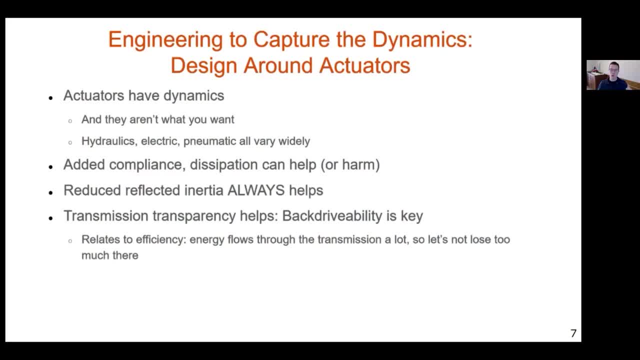 There are a lot of drawbacks to that, Like energy use, but they do get the performance out of it. Our approach has been focused on electric, because of the efficiency, because of the cost effectiveness of it, And I think that At least understanding the passive dynamics, or understanding the actuator dynamics and then integrating passive dynamics to help get the behavior that you want, is very, very feasible to to do everything we would want to do with these robots. 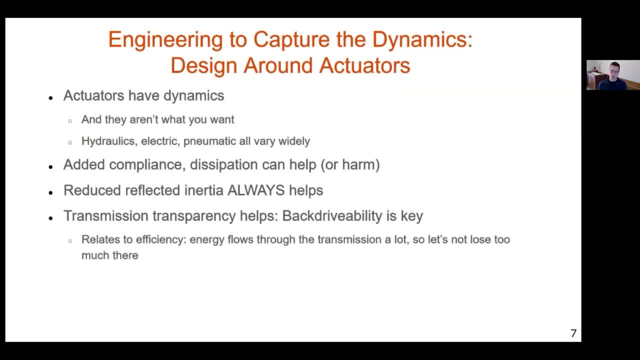 I guess Another thing to mention is muscles, And I think that's a really important aspect of the dynamic behavior of muscle is that it's not necessarily optimal for the behaviors that we want, And I think it's becoming more and more clear that the dynamic behavior of muscle is not necessarily optimal for the behaviors that we want. they may just be limitations of the biomechanical process that allows muscles to do work on the world. 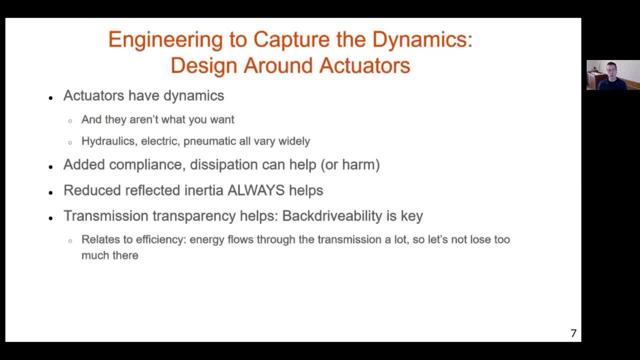 Certainly there are a lot of adaptations and animals with structures like tendons and the way the muscles are configured and shaped on joints that Clearly alter the behavior of the muscle, Clearly alter and vary the dynamics of the muscle. So it is absolutely an animal, is absolutely not all software, It is not something where you're sending muscle commands to have your arms and legs do what they want. 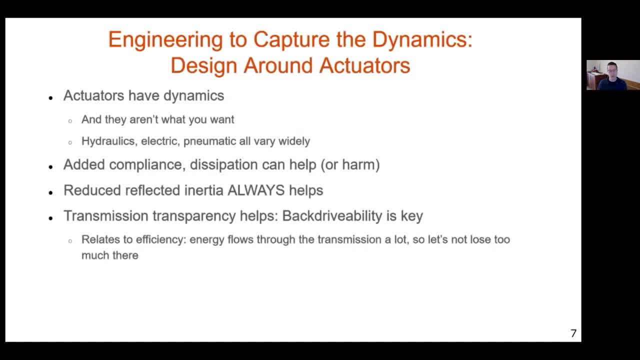 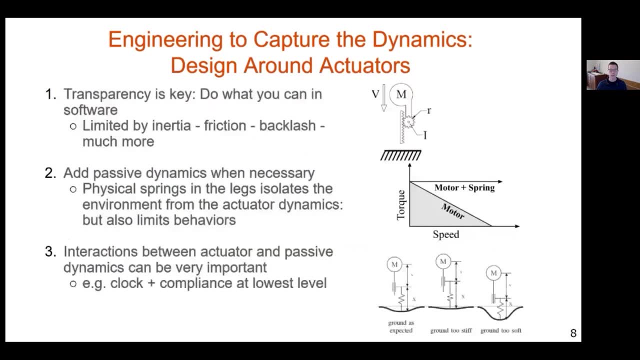 There's an immense amount of passive dynamics designed and built into all animals In order to create appropriate dynamic behaviors. Okay, so a little bit more about about this designing around the actuators. Transparency is key, and transparency I would define as, in software, you command a torque and in hardware, you get exactly that torque. 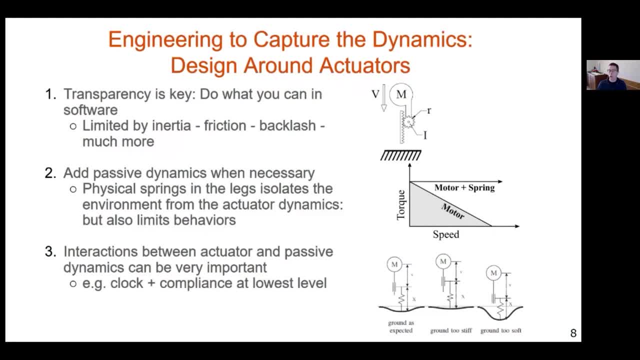 And that's at all frequencies, that's at all amplitude. So if you command 500 Newton's, you get 500 Newton's. if you command 500 Newton's at you know Oscillate between positive 500 and negative 500 Newton's, at you know 5000 hertz, you get it. and and obviously that's not possible because 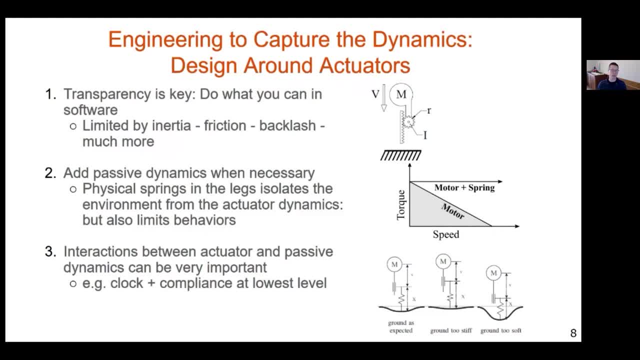 Of the inertia associated with motors and electrical dynamics and everything else. So, if you can, reduce your reflected inertia, make your motor rotor lighter, make your gear ratio smaller. Find a way to get enough torque out of something you know without having a big gear ratio. eliminate friction, have a completely transparent, you know, efficient transmission. 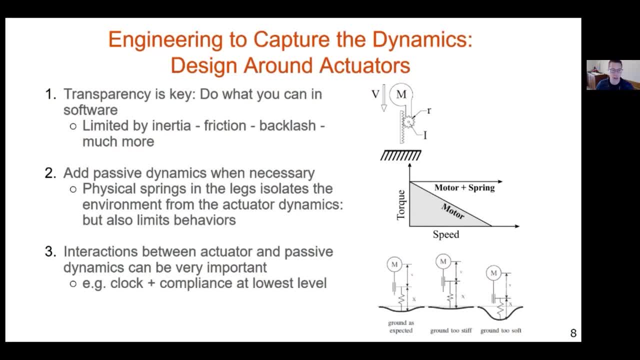 Things like cable drives. We got something like 93- 94% efficiency in the cable drive on some of these early robots. That's great. There's other drawbacks to a cable drive but a harmonic drive there 75% ish, something like that for friction and that can be really limiting if you're trying to apply forces to the world because you don't know what force you're applying. 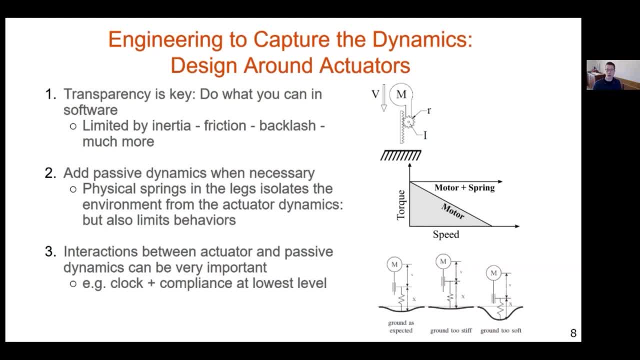 I'm getting a question from someone. What would I like to see from the future of electric actuators? the best way. so. ghost minitar is a great example of a direct drive Robot and at a very small scale You can do that. you can have relatively very low inertia and relatively enough torque to do what you want to do and get that robot to leap and jump and do all kinds of things as you scale up, especially to something the size of Cassie or digit. 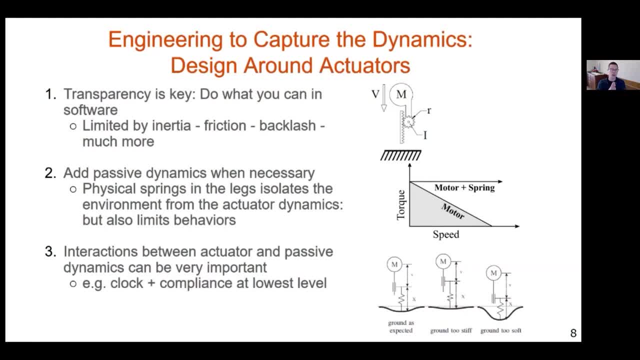 You know the the torque from your motor goes up by the square of the surface area that you're getting on your magnets. But the mass of your robot goes up by the cube because it's volume And so the larger machines. You just can't. You have to put a gear ratio in there. 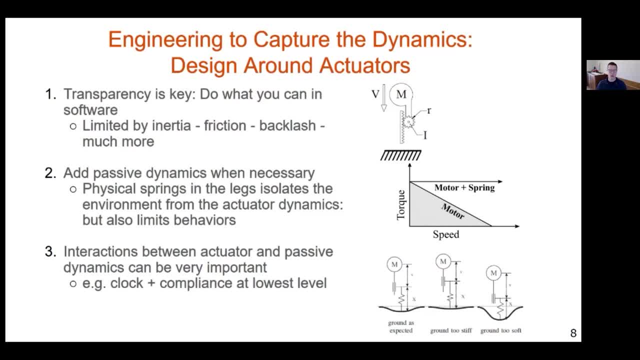 And that gear ratio gives you inertia, It gives you friction, It gives you a lot of other limitations And that's why we add the big physical springs on a tree, That's why we have springs on Cassie and digit. We also are handling, you know, the, the foot contact. How do you interact with the ground when you make contact? So a lot of engineering that goes into what is impeding our transparency. 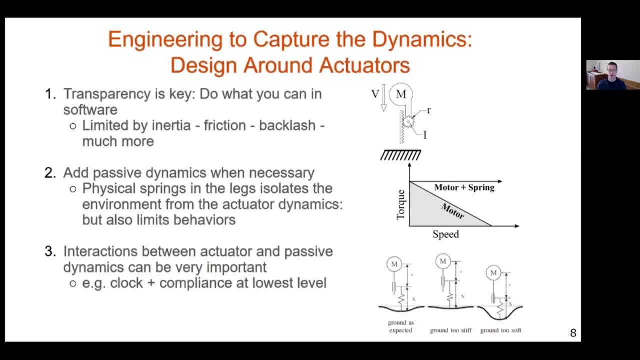 And so I. in my opinion, the best solution is to have transmissions that are Very, very efficient, Very, very low friction, meaning that you can command the torques that you want and you're going to get them. and then ways around the inertia problem, ways to handle the impact with the ground that mitigate the inertia. 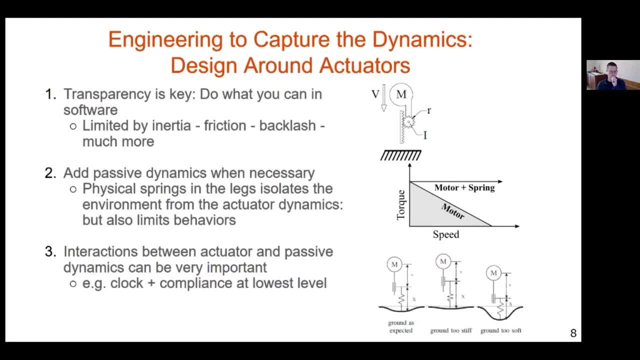 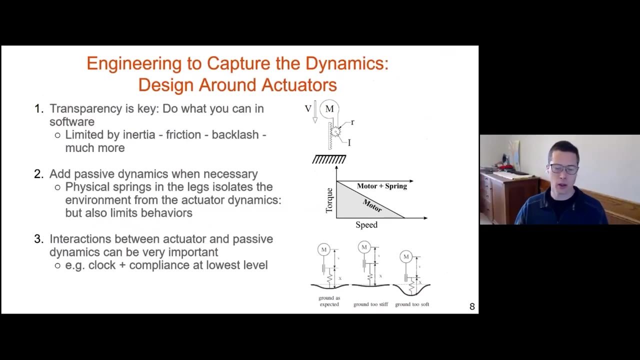 I don't know, It was just my current guests right now. Let's see What else can I say on this slide. I'll say that early on It was an interesting observation that If you have some sort of clock cycle, Say your controller is only operating at 30 hertz and I you know, obviously control systems can run at 24 kilohertz, at two kilohertz easily. 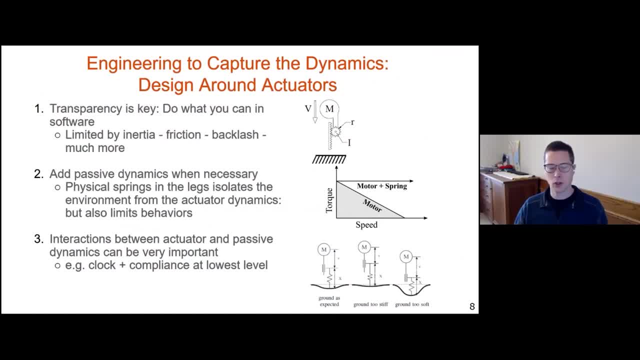 But you can't really perceive your environment. Sensors are always noisy, late and wrong, And so it's very, very hard to plan exactly what you're going to do through some sort of impact or contact with the, with the ground. But If you do things like have a clock based feed forward cycle, 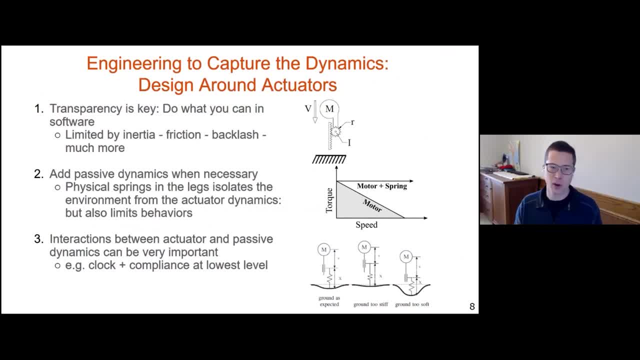 And kind of what you expect to happen and have that clock based feed forward plan in series with a big compliance. You know, we found that very self stabilizing. In other words, if you hit a little bit early or you hit a little bit late, or you hit ground but it's too hard or too soft. 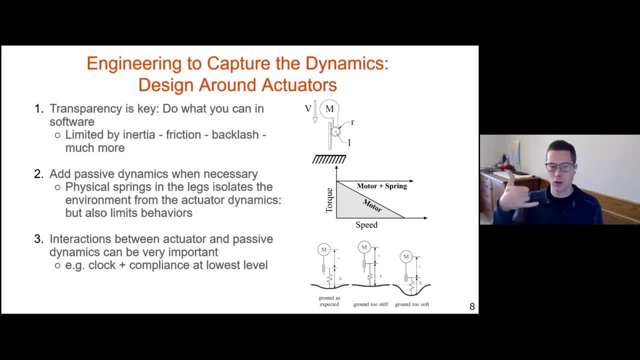 The immediate reaction just from the dynamics of that clock in series with the spring is is is stabilizing, it is going in the right direction. to cause your ground reaction forces in your center of mass motion to go in the right direction, Then you can react fairly. 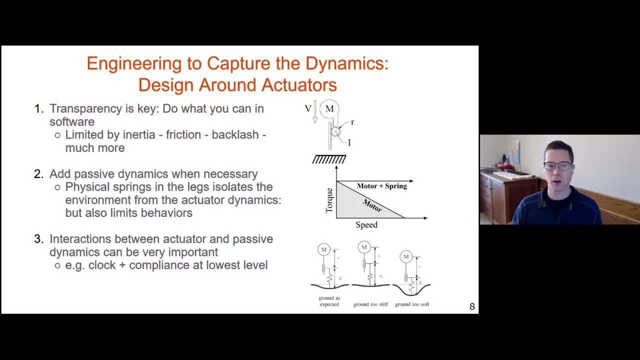 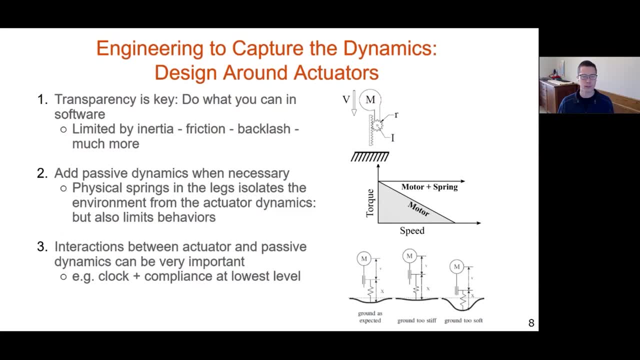 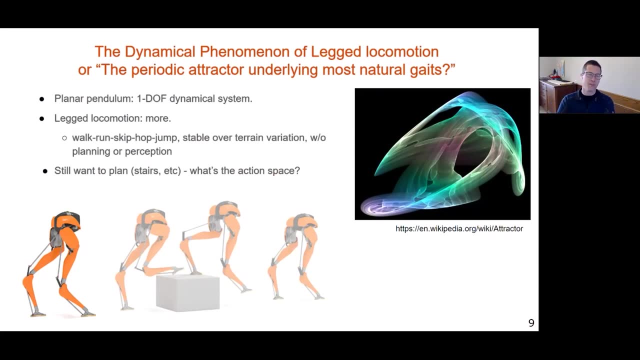 Slowly, but creating that stability as an inherent part of your system is is what's important here And boy, there's a lot to solve. There are a lot of science still understood. Okay, so I talked about the dynamical phenomenon of like a locomotion. Maybe another way to think about it is it's some sort of periodic attractor. 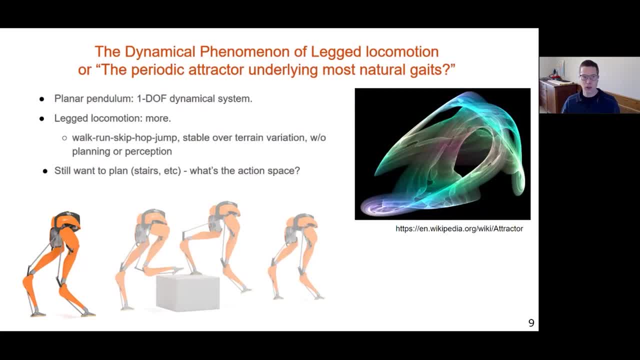 And when I talk about a pointer, pendulum or spring mass system, Of course that's a one degree of freedom system. There's really not a lot you can do to influence that System is just one degree of freedom. It is stable, It keeps time. 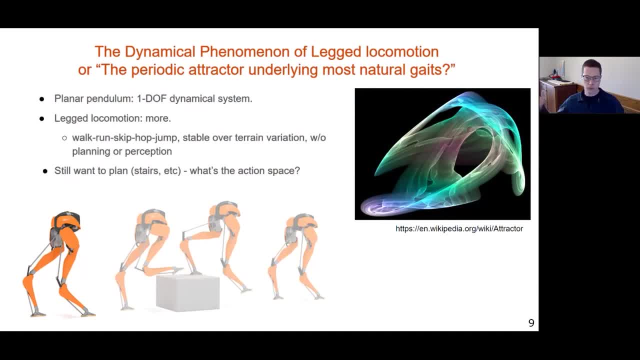 But I think, like a locomotion is many more. Maybe it's seven degrees of freedom, I don't know as a periodic attractor- And there's a couple of degrees of freedom in that periodic tractor. So instead of just the back and forth of a pendulum, 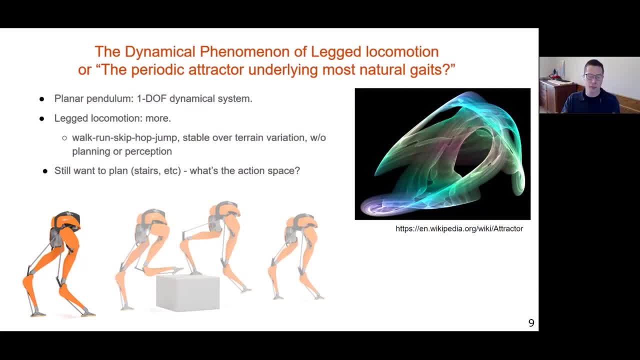 Maybe it's more like if a spherical pendulum had some stability region for it, but it's a five or six degree of freedom or more, And now you want to kind of choose. what's the action space, What are the inputs to the system that allow you to land on stable space? 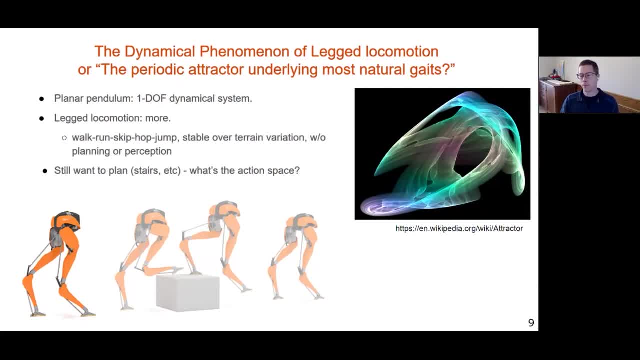 And what are the cycles that you would want in different directions? And one of them, for sure, is transitioning between the gates, and maybe that's how much energy you add, or maybe it's a how you change your clock cycle In order to scale between them, but whatever gate you land on is still stable, self stable, periodic attractor. just you've got this degree of freedom. 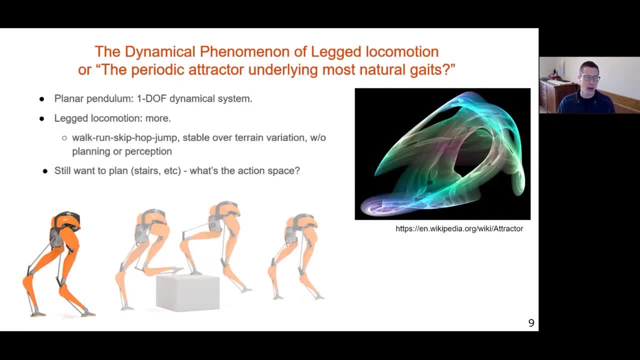 Now another one might be like stride frequency and stride length. you know, I don't know the answer really, But I picked up this cool picture from Wikipedia. It's what an attractor looks like. That's obviously more than one degree of freedom and we are kind of coming up with. 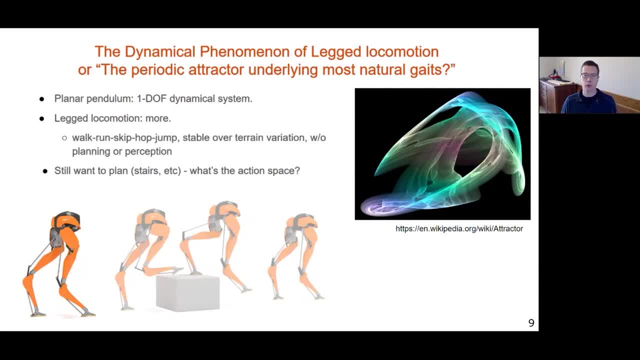 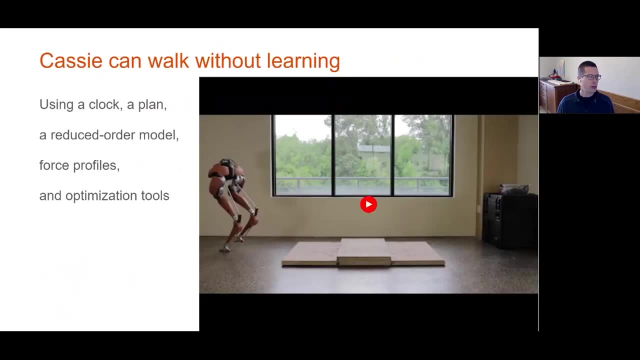 I would say incomplete and not quite correct- heuristics that get us pretty close and are able to start really exploring some of these behaviors. Someday we're going to have the complete picture of what this looks like. So just to start with, I want to point out Cassie Atreus- all of our robots can certainly walk without learning. 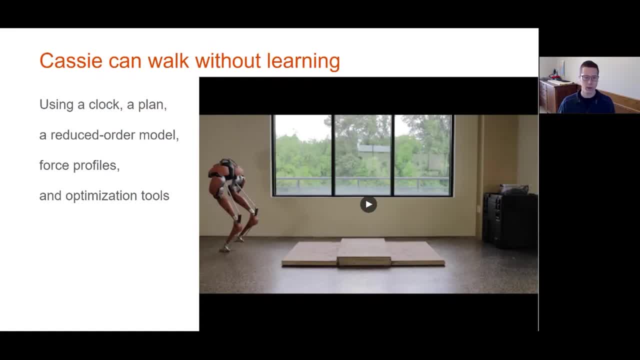 We have a clock cycle in them. That is kind of like our feed forward behavior. We have a plan. In other words, we know that, You know we want to go right foot, left foot. We, in this case, have no information about the world, but we can have information about the world And that's what the planning does. We have a reduced order model. 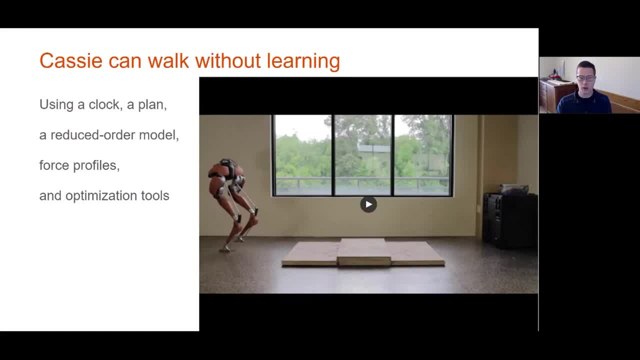 Inside that allows us to make choices about, say, where to place the feet in order to stay balanced, and an optimization tool so that you can Basically map this Very complex robot with lots of joints and more joints and more behaviors possible than the reduced order model enable, but optimize for your priorities so that you actually get close to what your reduced order model is saying. 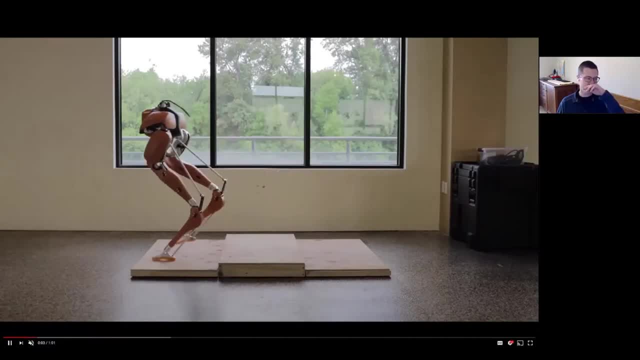 And so here's Cassie just walking over some unexpected terrain and handling it pretty well because of the transparency in the actuators. So you'll see that the robot maybe steps up a little bit, But at first, when it steps up a little bit, it's not going to be able to do anything. 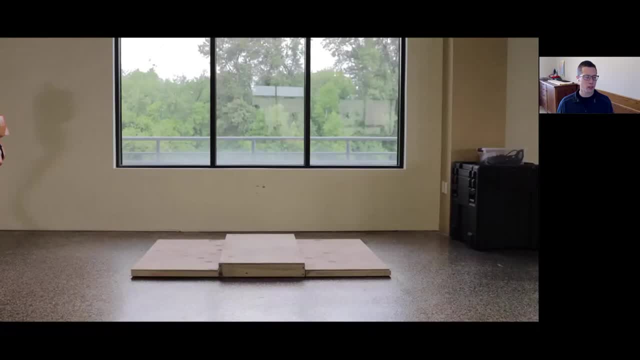 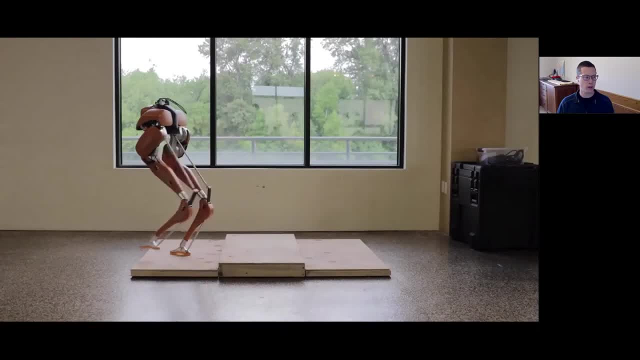 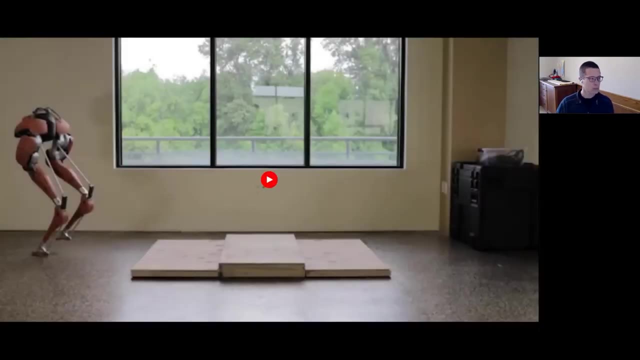 Then the robot walks up continuously. So you do wanna have some priority as well on your, on the force at your other position, that you're where you are. And that's what I mean by optimization tools. You've got several different goals. it's balancing between those goals, kind of trying to optimize for things. 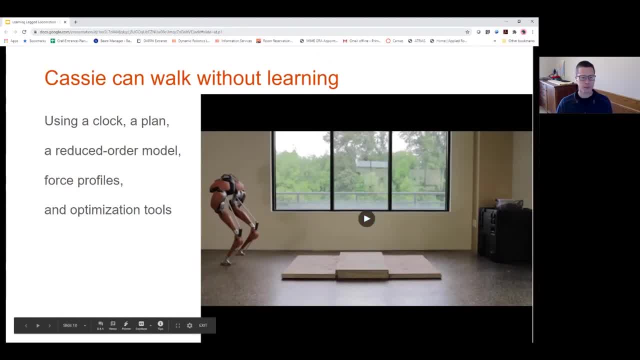 Dominick Kelly. Hey, Jonathan, can I ask? can I ask a quick question, But maybe, with respect to your point about legal locomotion being a dynamical phenomenon, can you comment on the sort of anxious pace that CASI does, even while stationary? 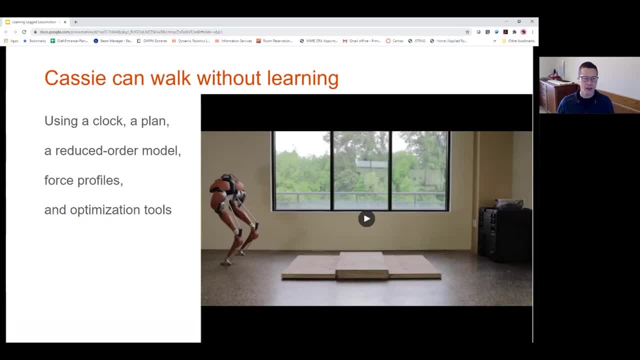 So CASI can certainly stand, but our controller has a clock as part of its foundation And so really, it's walking at zero velocity when it's stationary, because we turn on the walking gate and walking behavior And then we can just change its velocity and it changes its foot placement in order. 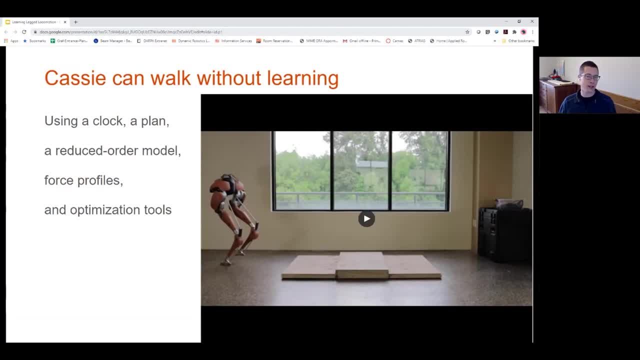 to go forward or backward at different speeds. That's all it is. I don't think that's necessary. It's just that's what our controller is doing right now. No, that makes sense, because you're just getting ready to steer it. 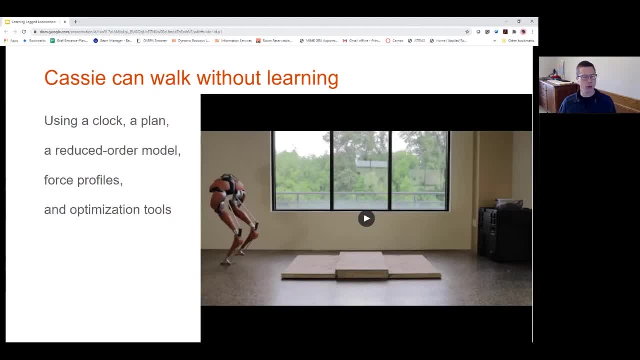 You know you're getting ready to drive, it right? Yeah, And so this is very manual, right? So the operator is saying on his controller: okay, turn on walking gate behavior, Okay, change speed forward, backward, et cetera. 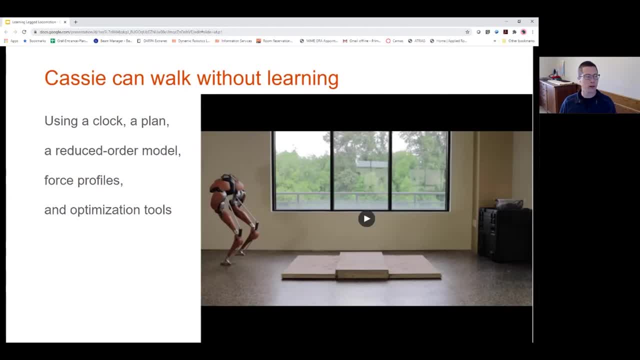 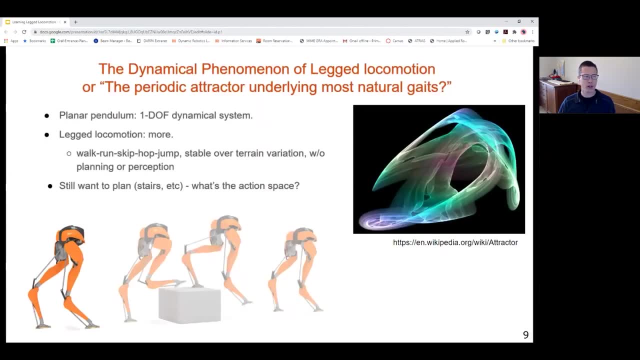 There's not a lot, There's not a lot deeper than that. that's going on here. But what I would like to be doing is, you know, going towards this kind of periodic attractor, which probably has a zero energy point too, that's also stable, which is standing. 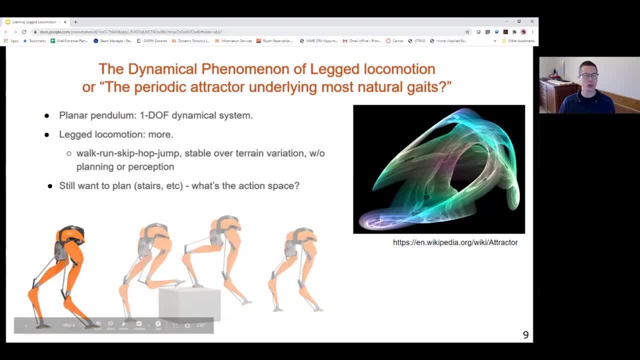 which probably looks a lot like zero moment point control. It's just using ankle torques in order to stand in one place, But that, I think, is on a continuum, along with the walking, running, hopping, skipping, jumping and all the other things. 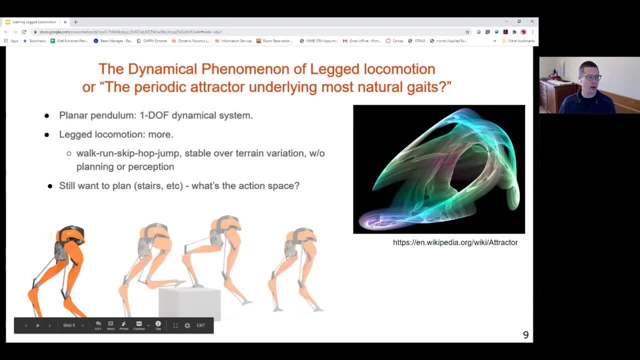 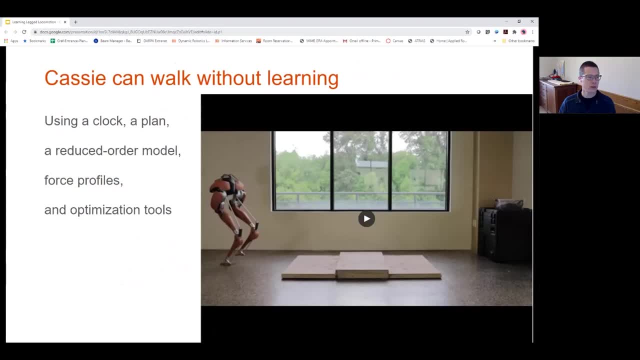 I just don't think we've figured out how to implement that. well, on hardware Got it. And then there was a. there's a question In the chat following mine about slippery, slippery surfaces. How does it behave on oiled floors? 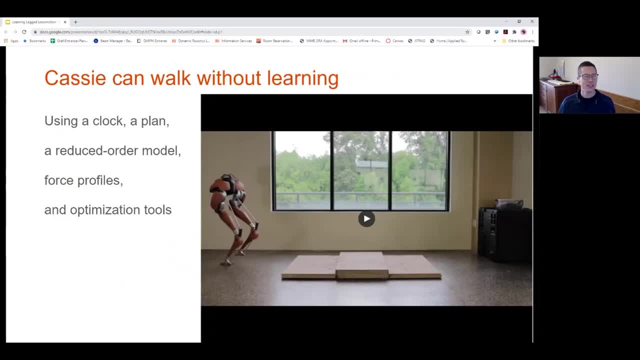 Same way as a person just falls right over. So we we do have kind of an estimate of the friction cone and that informs things. like one of the early lessons we learned is: you don't use a toe switch, Just you don't know when it's on the ground. 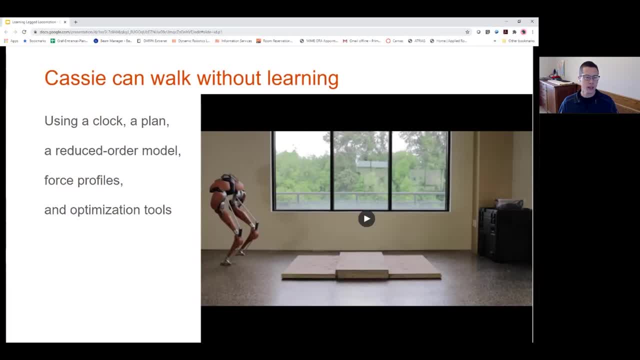 You have some stochastic estimate of when your foot's on the ground or not. If your foot is in the air, you kind of you want to be placing it on the ground, You want to be placing it in a particular position so that when you do land, 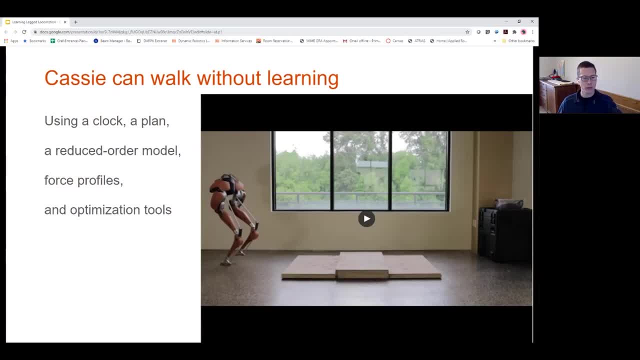 your foot's in the right place. But then, when you're on the ground, when can you start applying forces in the X, Y, you know, in the four apps? When can you rely on the fact that your foot's on the ground and you can apply? 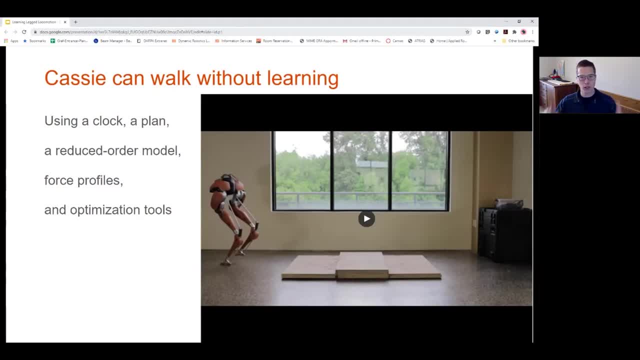 lateral forces. It's really only when your vertical force starts to increase and we have some estimates of the friction cone, And so there's a big gray area, the first and last 10% of of stance phase. You don't really know. 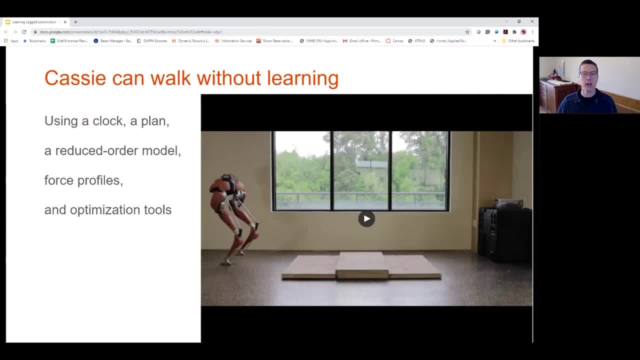 And your controller doesn't really know or rely on whether you're on the ground or in the air. So there's kind of a point where the swing phase and the stance phase are kind of they're kind of separate controllers but kind of tangent to one another. 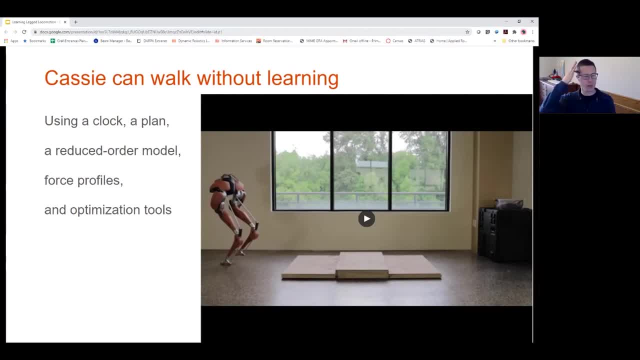 So they're both kind of trying to do the same thing for that 10% overlap at the beginning and the end of stance And the behavior changes a fair bit if you modify your estimate of the friction cone. So that's again something that kind of fits into. one of the optimizations is an estimate of 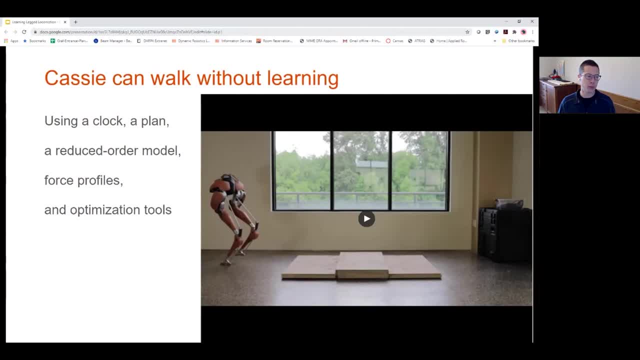 what you think your friction cone is. So if we wanted to walk on ice and we were able to perceive that it was ice, uh, that's what we would do. We would modify the friction cone. The robot would likely take much shorter steps because it knew it would not be. 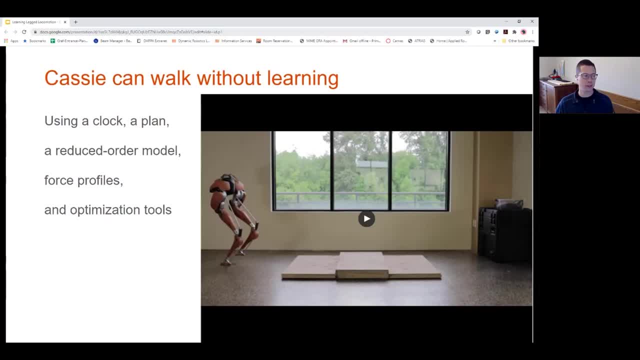 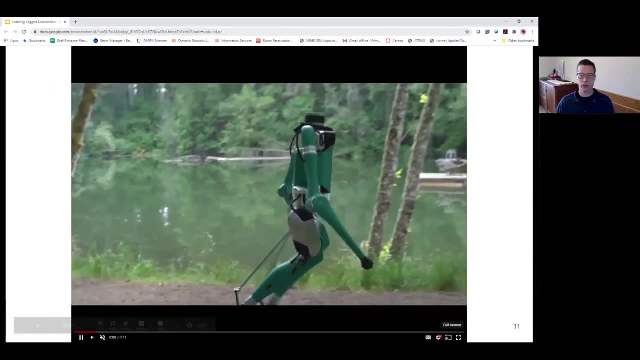 able to take a big step and rely on, on that friction, uh existing All right. So, uh, I also just want to show a couple of briefs. These are the only two videos I'll show a digit, uh, walking around outside. 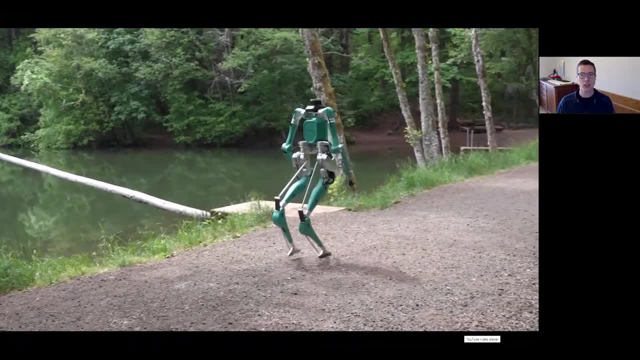 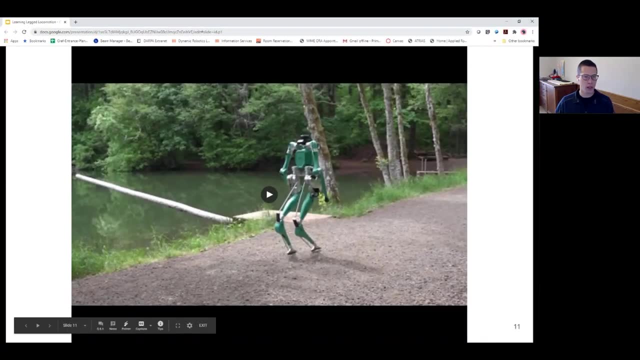 It's the same configuration of legs as Cassie, because physics is still true. The reasons we designed the legs the way that we did are still the case, Um, although there There are a lot of differences- internal, uh, between the Cassie and the digit legs. 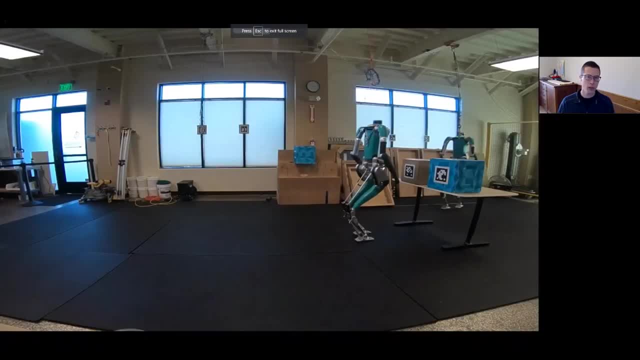 And so, building on the, you know the, the locomotion, which we really have not been paying a lot of focused attention to because we've been really working on incorporating, you know the using the arms to swing- uh, using the arms to manipulate the world. 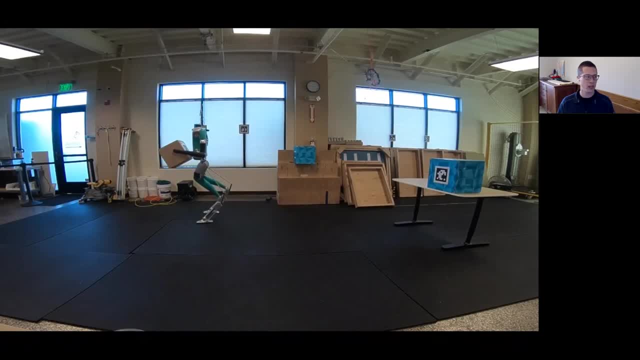 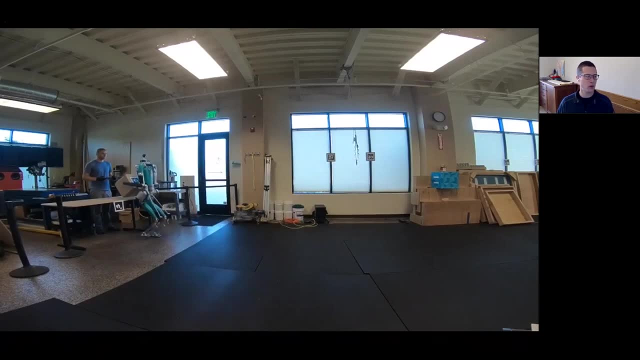 and balance the robot with the different masses of things that you're picking up, catching the robot when it falls, reorienting to get back up, starting to add in perception. The robot here is using those QR codes to uh identify where the table and the box and 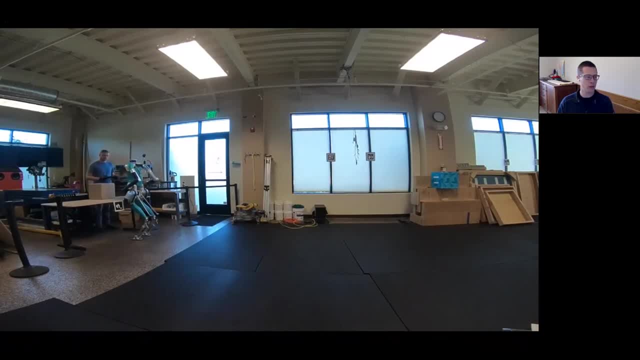 everything is in the room, uh, using the LIDAR to avoid obstacles. So starting to build a much bigger stack on the foundation of, uh, the basic locomotion that we've got. there's so much room for improvement in absolutely everything that the 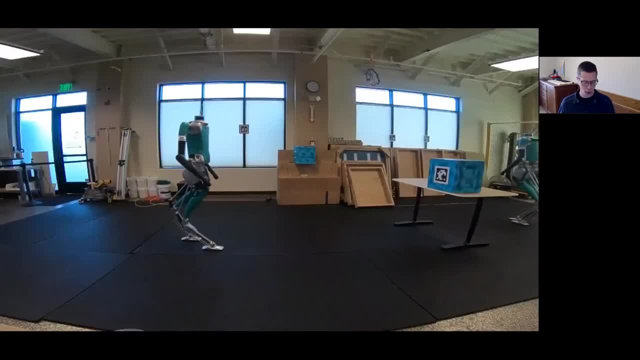 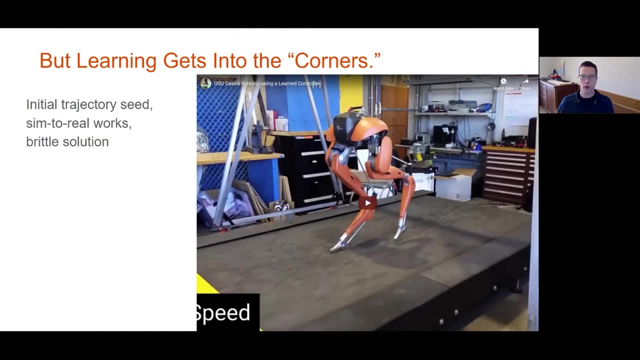 machine does. Um, we really have to pick and choose what it is that we're going to be doing. So the thing that's nice about learning, as I mentioned earlier, is it gets into the corners, I would call it, And what I mean by that is that when we're controlling digit, when we're controlling 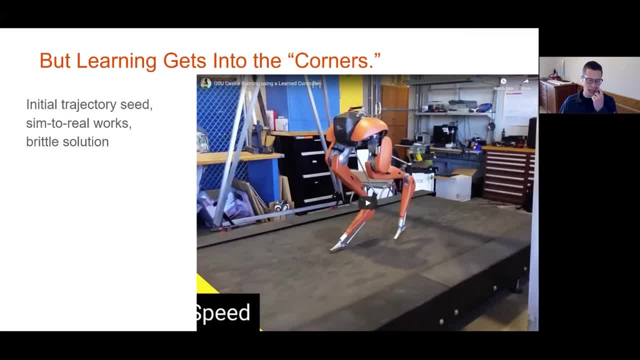 Cassie, we're relying on some reduced order models and, uh uh, that constrains our behavior. There's there's a real constraint, but if we did, we in this video, I'll show we. we started with an initial trajectory seed, and this trajectory came out of Cassie's. 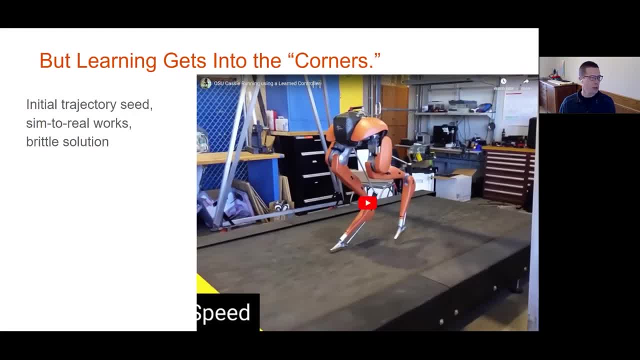 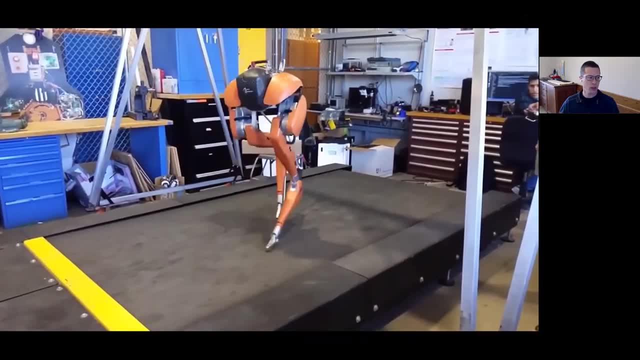 uh traditional controller that we'd already created, Um, and we tried it on the robot for the very first time and and it worked. We were able to do the simulation to the real transfer. I think a lot of that has to do with the correlation between the robot behavior and. 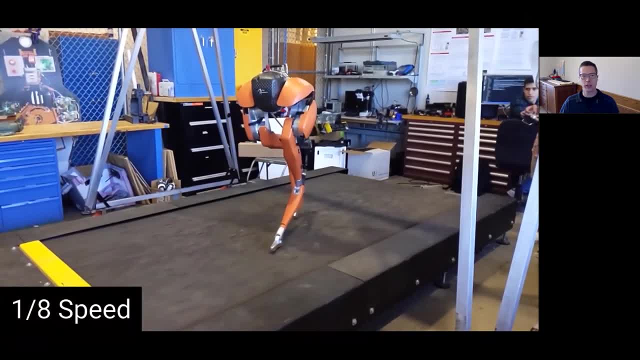 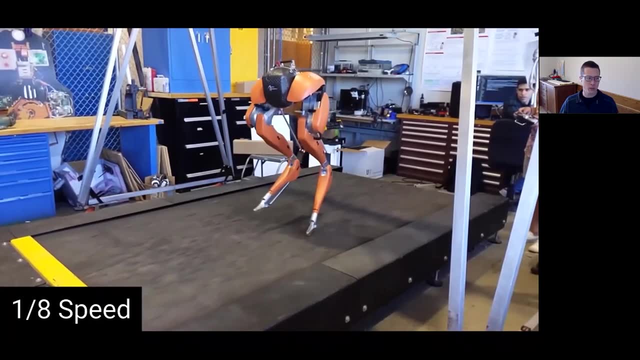 the simulations behavior. It also has to do with the self-stability of kind of the behavior we're trying to create. where we are, the robot is roughly a spring mass system So inherently it does have A lot of those abilities that that we talked about early, that I talked about early on. 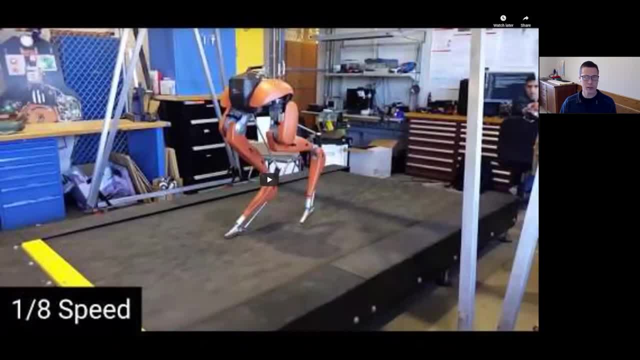 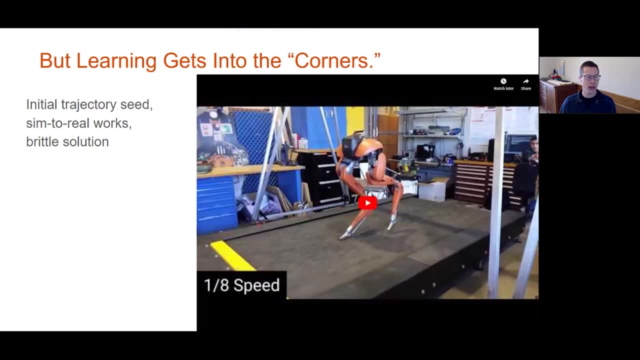 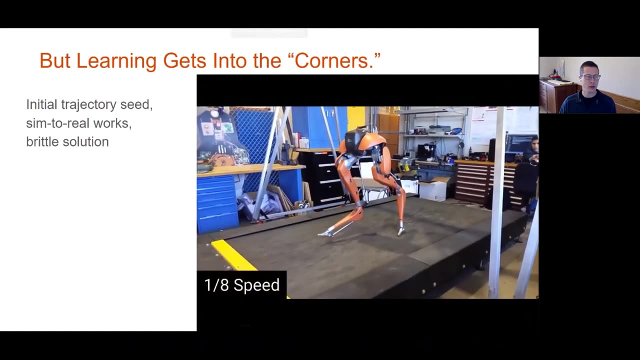 in this discussion, Um, but we're not really explicitly utilizing them. We're kind of accidentally utilizing them in this and it is a pretty brittle solution. This running gate, I love it. I think it looks very biological, Um, I really like it. but you know, it does fall reasonably easily. 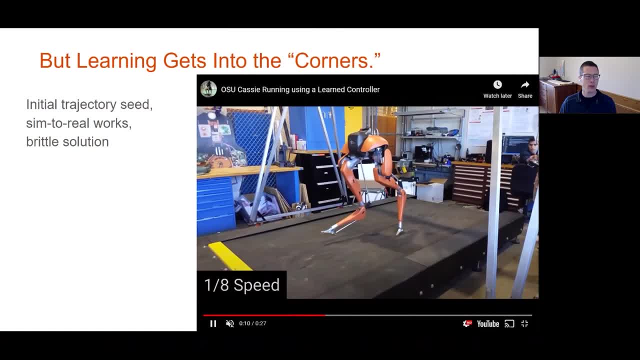 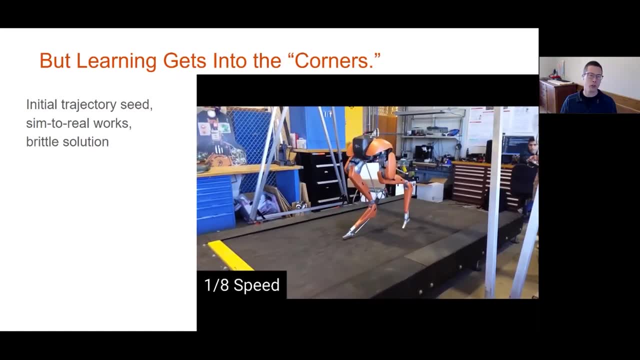 It's very sensitive to the friction cone on the feet right there. So this behavior worked on the treadmill, But when we did it on the road- even the crown of the road- it was falling sideways. Um, it would twist its feet when it uh, the feet would just slip and twist on the ground. 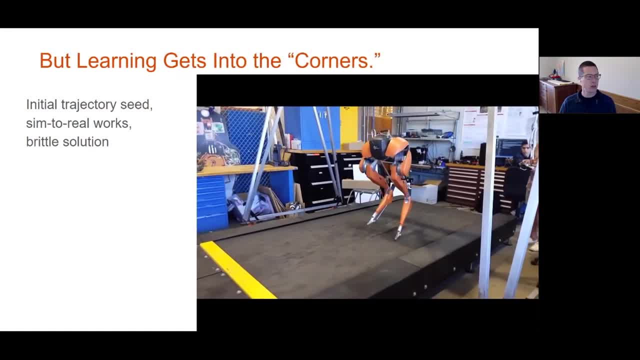 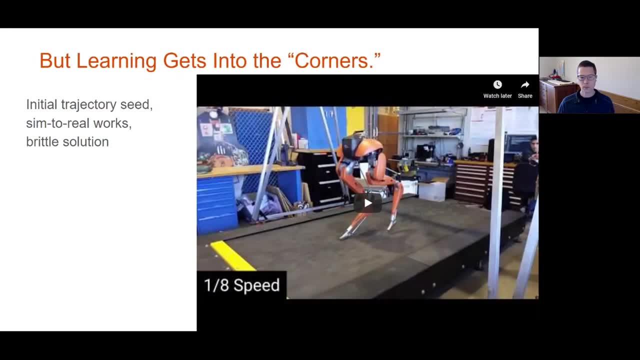 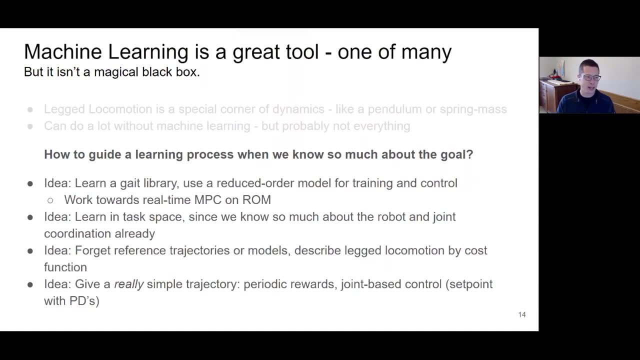 when we were on pavement and this would fall over. So this particular initial idea kind of got pretty brittle. but what a dynamic behavior we couldn't achieve without learning. So, um, I'm actually taking longer than I thought to talk. I'm going to have to move, move along a little bit here. but uh, the question is that how? 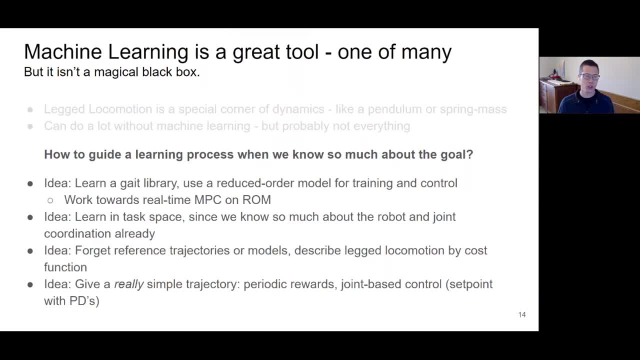 do we guide the learning process? And, and you know there's, there's something that's going on where people are going to be, um, trying to figure out what to do and what to do differently, And you know, I mean, I'm a dinosaur. 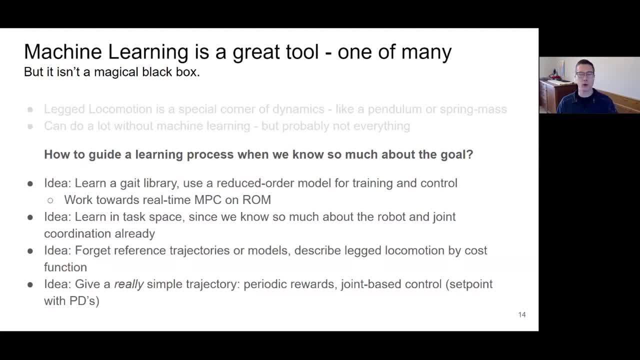 I'm going to take all my time. You know, I think it's like you know, like what you're going to do, But when you're in the room you're, you're probably learning, right, Not that you know. you're going to have to explore what you're going to do. 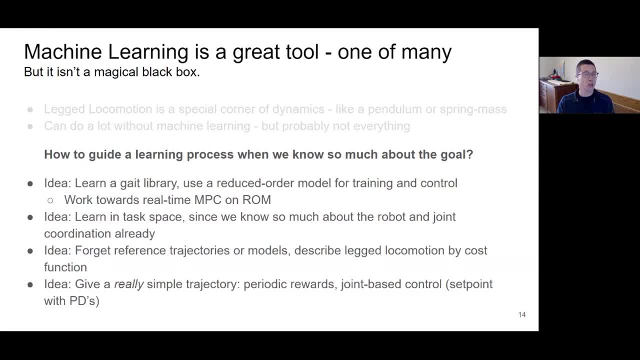 And so Um. so this is this is the first one, And then um, but then there's also the next one, which is um. something you know that I'd like to talk about is um. how can we, you know, change our learning patterns on the field? 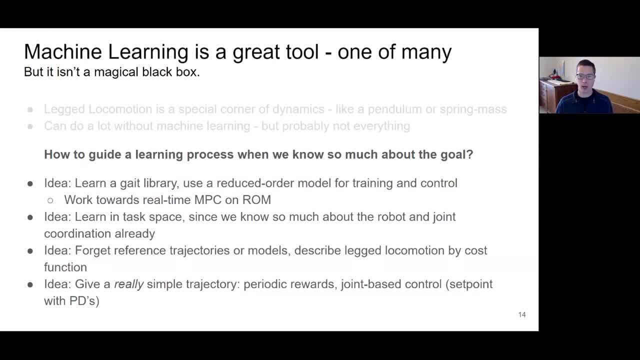 jump, But working towards having real-time model, predictive control using that reduced order model. Now the next idea is: let's learn in task space, since that's the common language. What should the feet be doing? What should the center of mass be doing? We already know a lot. 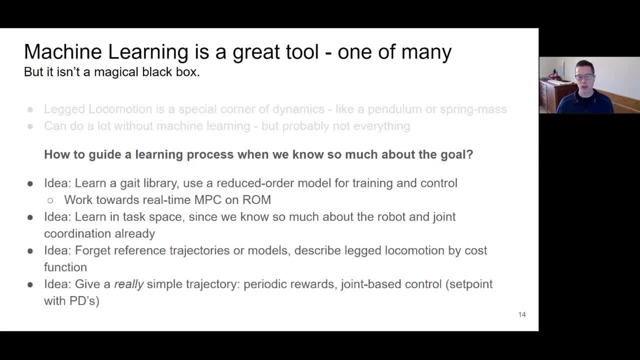 about the robot and we already know a lot about how to coordinate the joints. So why would we relearn how to do all of that and put the burden of the inverse dynamics and inverse kinematics on the learning system? We can just put that in there and learn in task space. 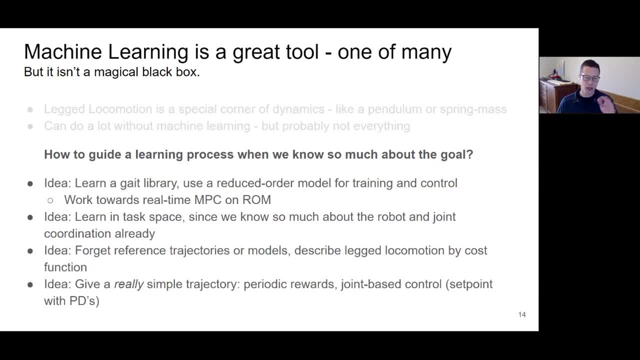 And another next idea is: okay, forget reference trajectories, forget even models. Let's see if we can describe everything we know about legged locomotion through the cost function. That gets some interesting results if you're very careful about it. But then kind of back to a little bit. 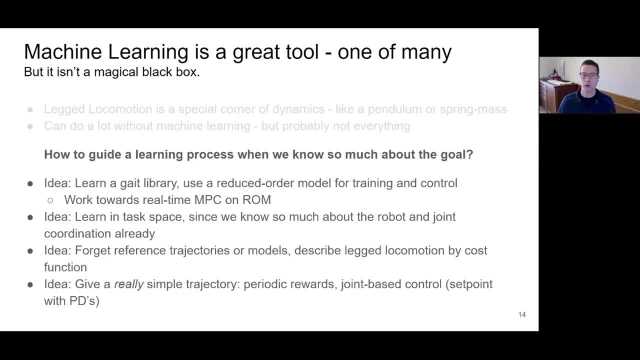 of the middle ground that clock seems to be really important for periodic behaviors. Can we give it a really simple trajectory which is just a clock signal, basically, but describe legged locomotion by the cost function? and where do we get with that? 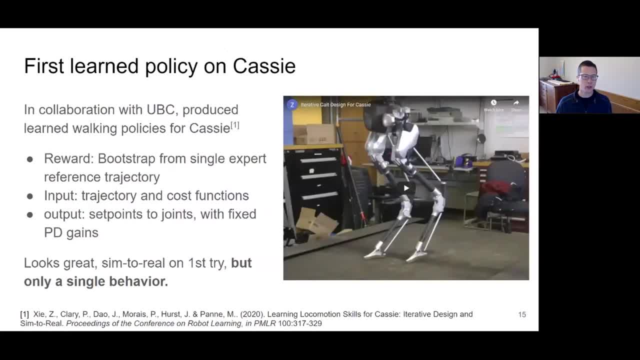 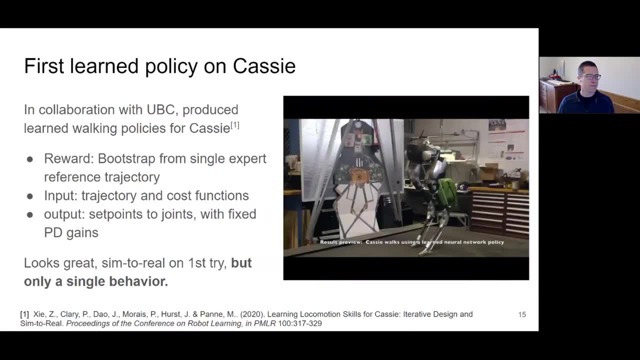 So this is the first learned policy on CASI in collaboration of Michael Van de Pan and the University of British Columbia, And kind of like the running behavior I just showed, it's bootstrapping from a single expert reference trajectory. It's just giving it position. 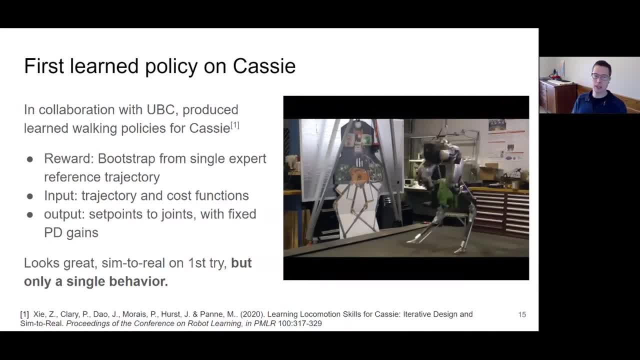 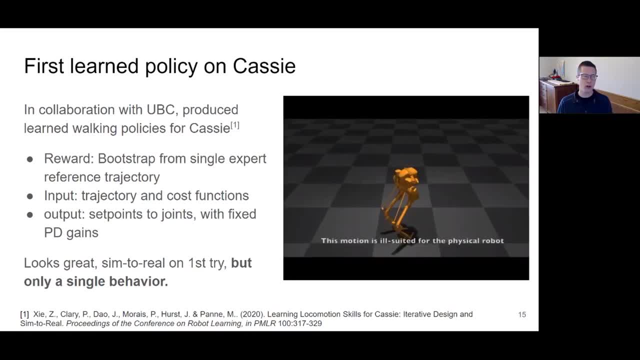 trajectories, which, in my opinion, is a very, very incomplete description or even hint of what's important, Because certainly, if you hit the ground a little higher, a little low, or you have a really different environment that you're encountering, you don't want to be running that original. 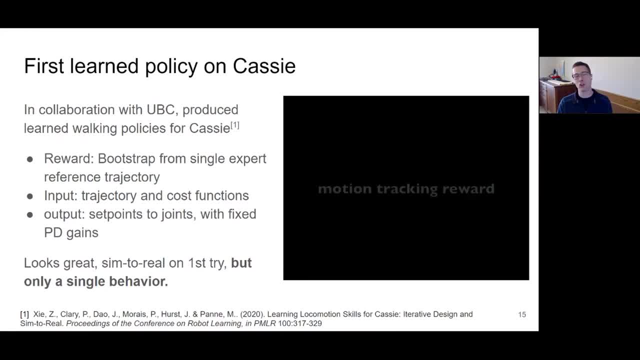 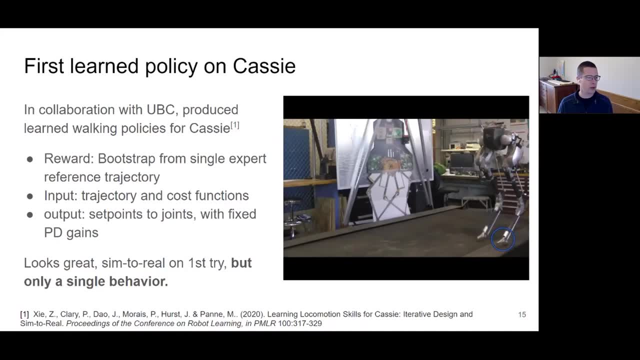 trajectory at all. That would be a bad choice, So it's bad information to bootstrap from. Nonetheless, we were able to get some pretty good results, but only for this kind of single behavior we were creating, And it did give us some interesting stability and robustness. I don't 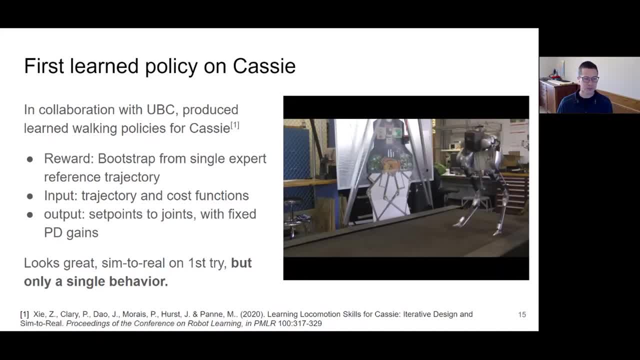 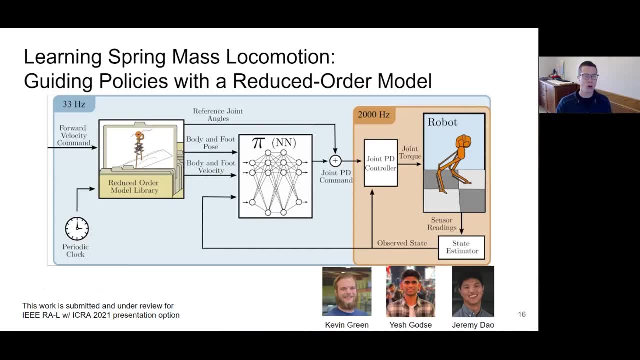 know why, but it did So. the next idea I mentioned: let's use a reduced-order model. Let's create a whole library of hundreds of different gates that come from, or are inspired by different gates from, the reduced-order model, And here we're giving it a lot more information than just trajectory. We're. 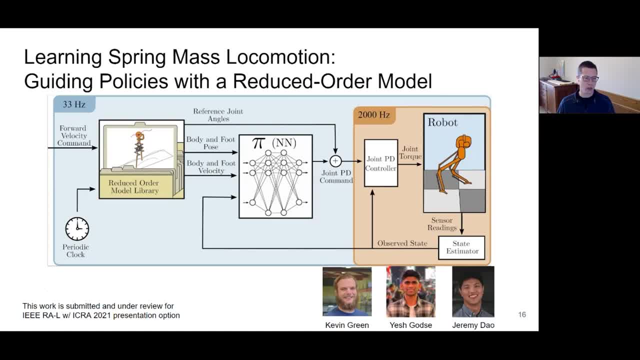 giving it the pose, yes, but we're also giving it the velocities. So we have an idea, then, of the forces that are being applied, because that model has those physical springs built in, And then we are, in this case, just commanding, So we can actually see the set points to the individual joints. The individual joints have their own PD. 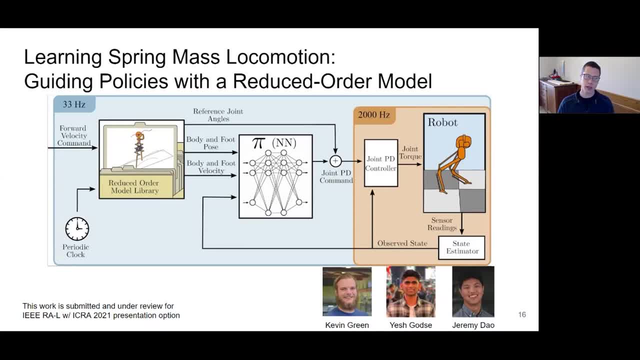 controls, that is known by the control system, And so this is sort of like a really fancy clock in series with some compliant behavior. The proportional gains in the controllers and the physical springs on the robot are a compliant behavior. that are very approximately something like the spring mass behavior. 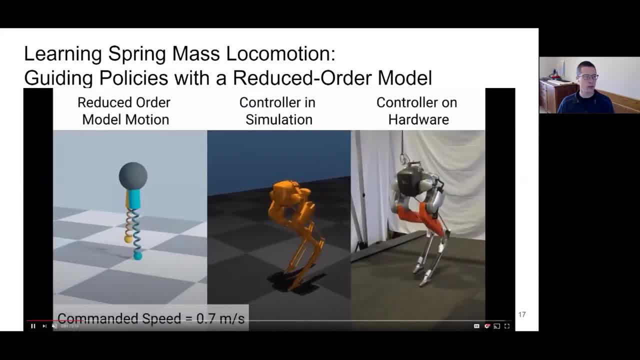 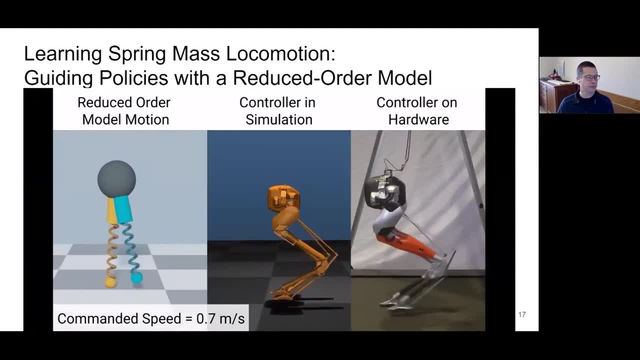 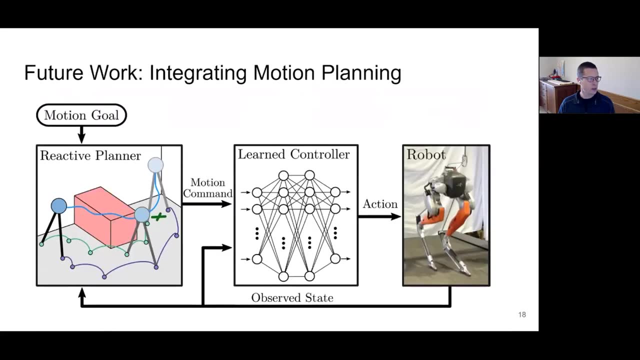 And this worked. This worked pretty well. just show the clear correlation between what the reduced order model is, showing what the simulation did, and then what we were able to do on the hardware. So this continues to be work in progress. It's aiming for IEEE right now. 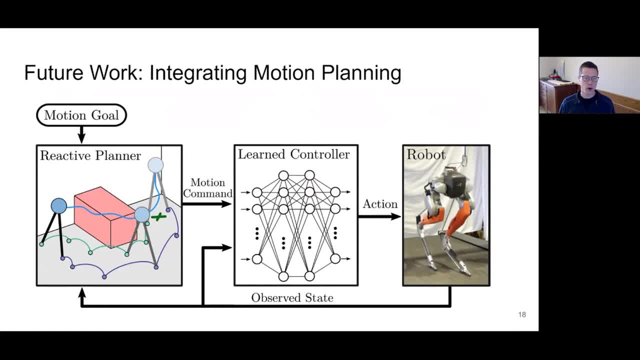 Now the next step with this is, instead of having a gate library, do something that's a reactive planner, something that has some perception of the world, chooses what it's going to do at the reduced order model level and then has the motion command. 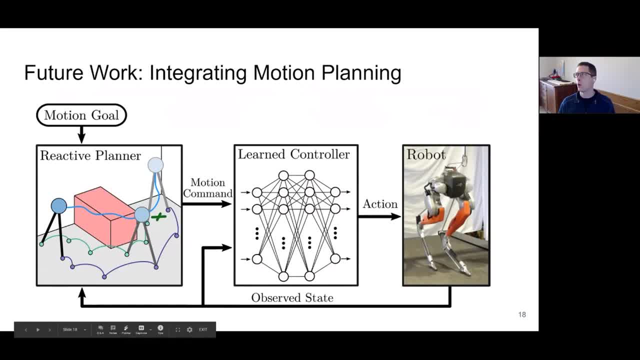 I don't know if I would even call it a motion command. It's more like: what is the state of the reduced order model? What forces, what is the set of dynamics that you're trying to create If the foot is about to impact the ground? 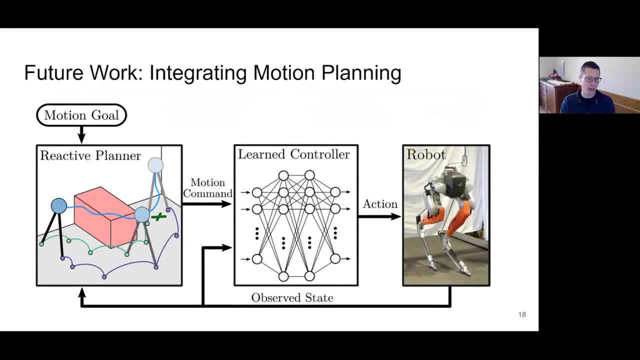 where should it be Approximately? what force do we want to be applying at the given point in time? And if the ground impacts the foot at some point, how do we want that foot to react? What kind of impedance would we want it to have at that point in time? 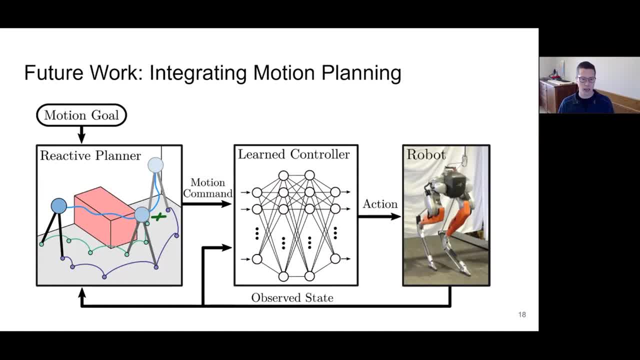 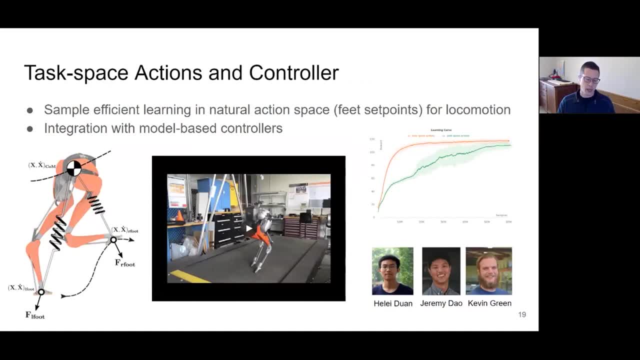 So that's a lot more information than just a position trajectory, because we are creating a dynamical behavior here. OK, so then the next idea I mentioned: why would we learn all the joint coordinations independently if we actually have a lot of information there? 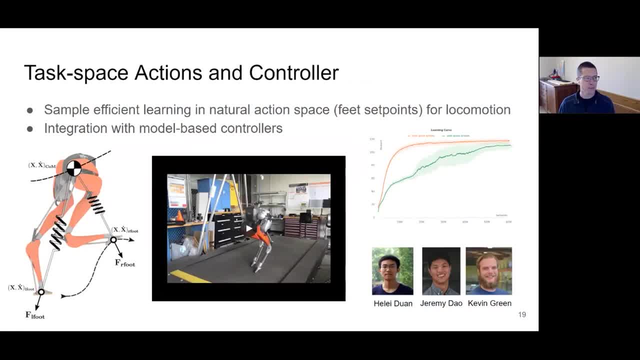 And, sure enough, when we learn in task space using these reduced order model kind of thing, it does learn a whole lot faster. It doesn't have as much to learn And it is significant And it's successful in doing some nice walking games. 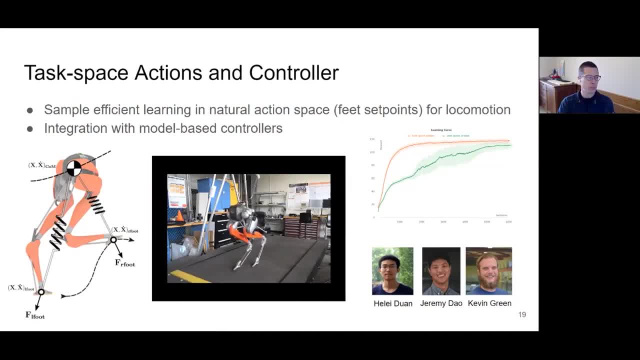 This kind of looks a lot like that spring mass behavior, but it learned it pretty quickly. So I think there's a lot of promise here too, And I don't know that we, the inverse dynamics, the inverse kinematics that we calculate for the robot. 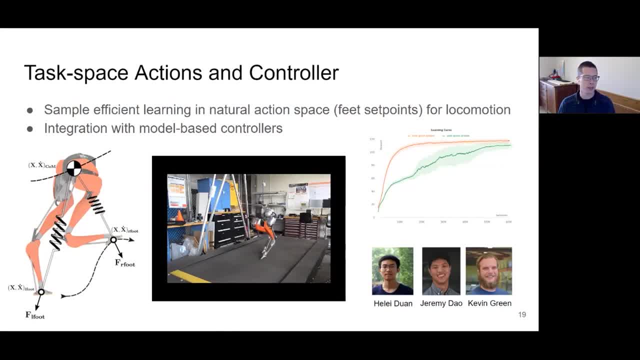 are certainly not perfect, because there's a lot of unmodeled dynamics going on in the hardware, But this is showing that we're able to sort of split things out in terms of how we tackle it. We're able to sort of split things out. 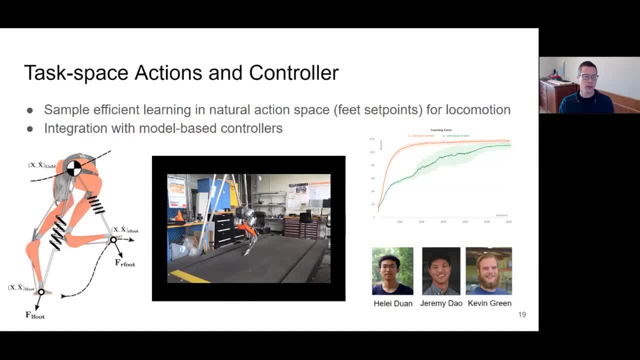 in terms of how we tackle a particular problem. This is just a small part of the overall control system, And when we're learning in task space, we're speaking a common language that works with any sort of model based planners or controllers. It also can speak with a separately learned policy. 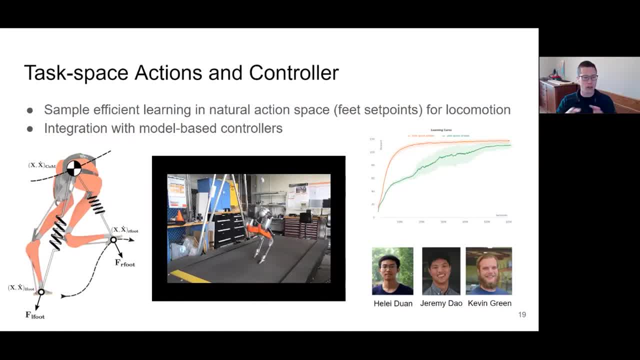 which would do all the inverse- kinematics for example- And so we're kind of choosing to have a control hierarchy that differentiates things out, so that the learning problems are much, much smaller And so we can get more precise or accurate representations in their very small domain space instead. 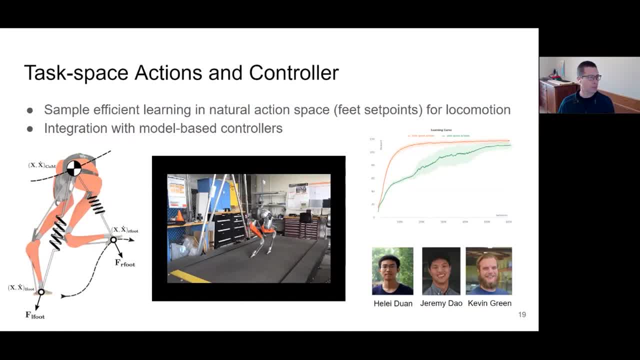 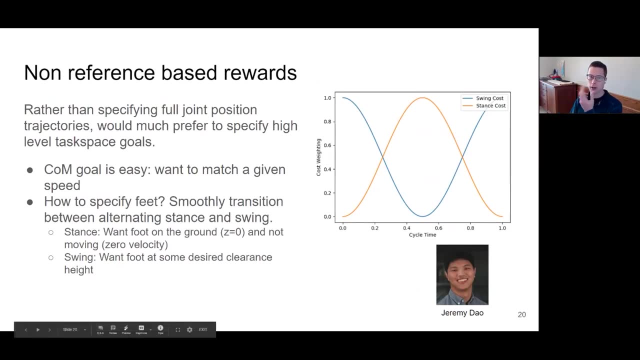 of trying to approximate some very, very big set of dynamics. So I think that's the power here- is just splitting it out into a series of much smaller and more feasible problems. Now, rather than maybe a trajectory or reduced order model providing dynamics guidance, the question is: can we? 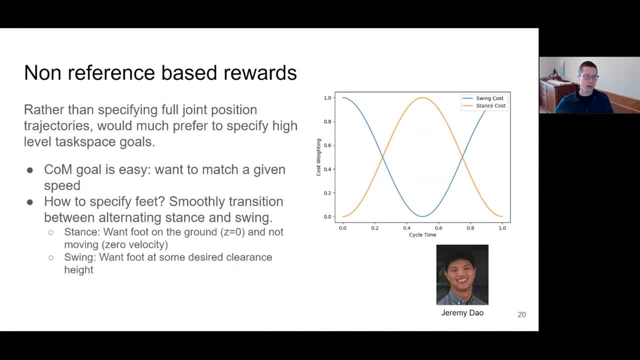 actually do the same thing with the same behavior we want, with really good cost function. In our lab we've done a lot of time, spent a lot of time kind of writing down what are the first principles, What is lag and locomotion? 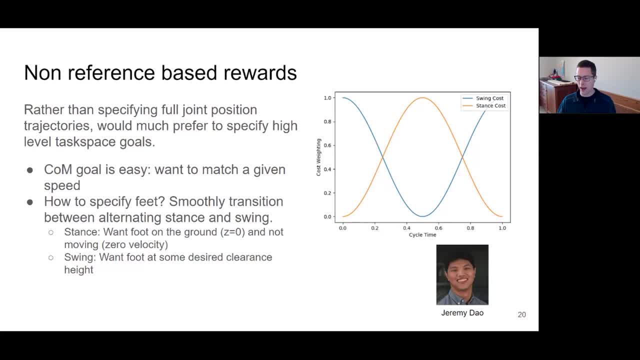 And it's tempting to say, oh, the spring mass behavior captures it, But it doesn't. It's just that that happens to be a model that gets close to what it is. But what is factually true about it? There's a lot that we can say about it. one foot. 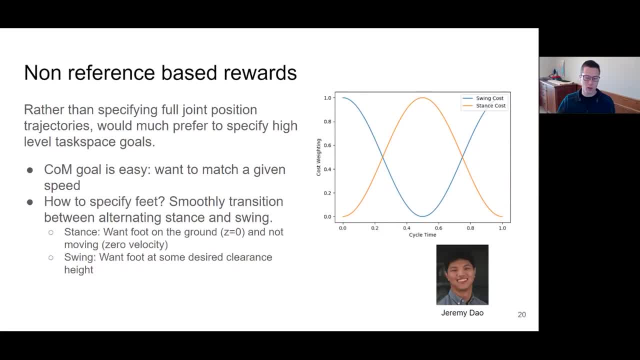 on the ground at a time, Or what's the, The smooth force trajectory that you would want to see, And we write a lot of that down and then try to put that into the cost function. So starting it's really challenging. by the way, 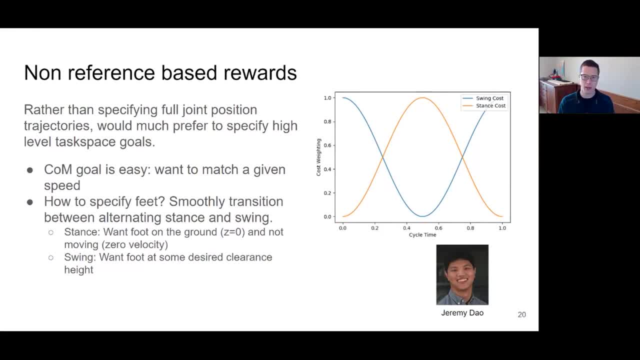 To start with physics-based stuff, what we think about how lag and locomotion works and translate that into cost functions that are in the language of machine learning. But we made some progress, We got somewhere with it, And here is a non-referential. 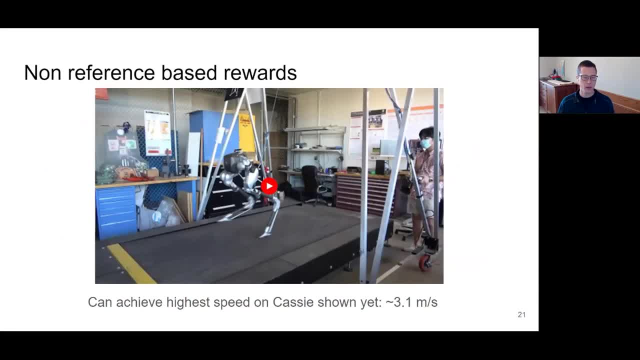 And this is a non-referential, which is a cost-based reward. No trajectory, no prior behavior that we gave it, Just describing it in terms of the cost functions, And this was we got the highest speed we've been able to show. yet 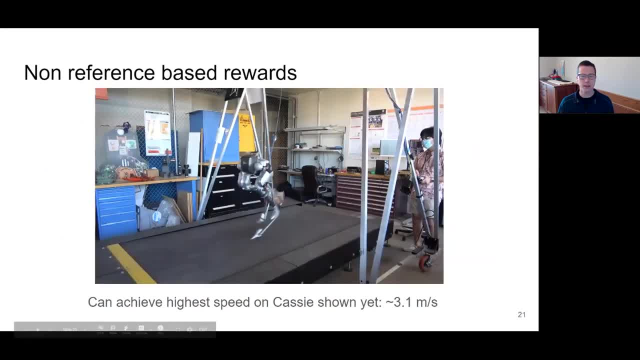 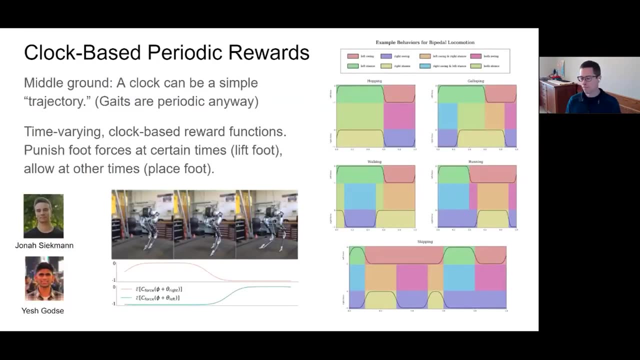 This is actually faster than the running gate that I showed at the beginning. I like the running gate, but this is faster, so Not too shabby, All right. so the next idea. All right, we are describing all of our behavior. 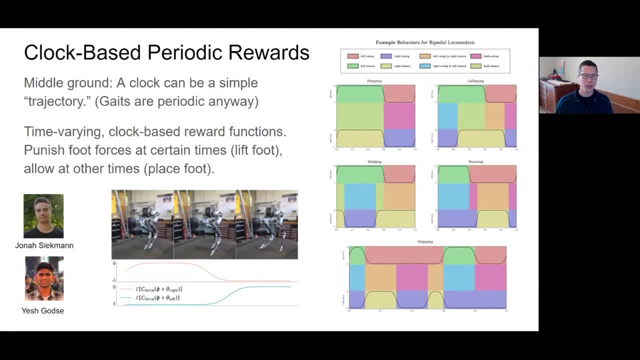 through cost functions, But kind of pick a middle ground here. Let's give it a little bit of a hint, a little bit of information. We don't actually know what an optimal trajectory should be. Maybe the reduced order model is kind of too constraining. 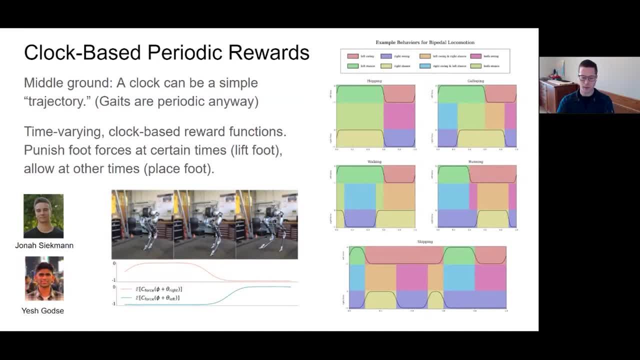 Or I don't know. we could do it in a much more computationally simple way, And so that's what this is. That's what this effort is: It's choosing a set of clock inputs that are very easy to modify, that are very convenient for the learning policy to utilize. 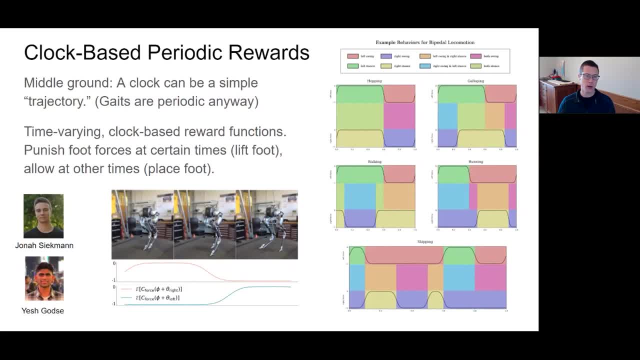 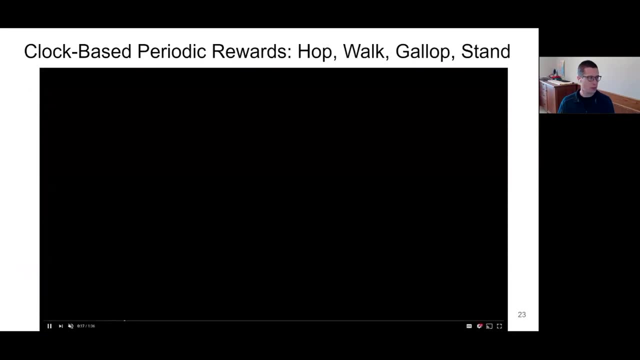 and much, much more computationally effective than using a reduced order model, And we were able to get some really surprisingly good behaviors out of this, Just choosing the duty factor of which foot is on the ground and when. And here's some transitions: 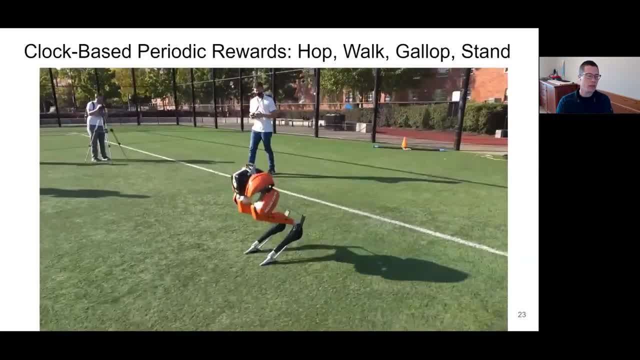 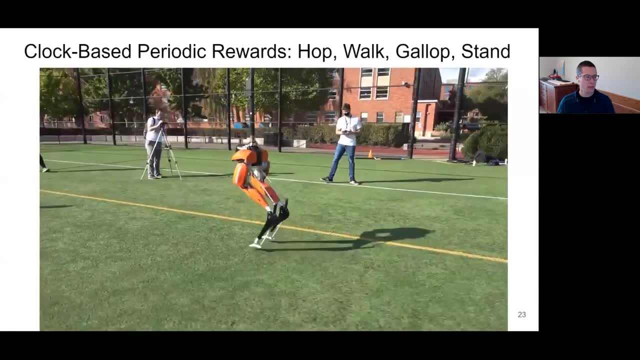 This is the first time I'm showing these videos publicly. Some of these results are just from the last couple of weeks. But here's Cassie hopping, And it'll do a transition from hopping to walking gait and then do a little bit of galloping and then. 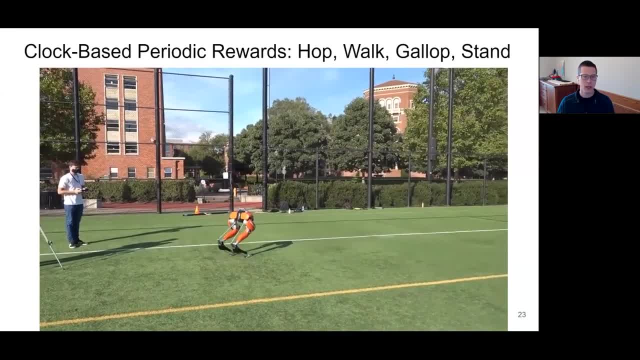 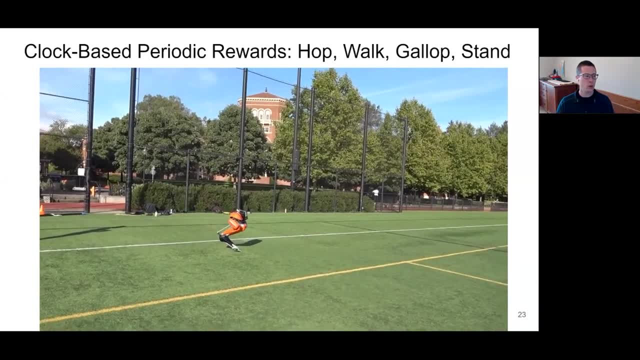 back to a stand behavior. All of these were learned in simulation and then tried on the robot. There's no online learning with the robot. All the learning is done offline. All right, let's see if we can get a little bit of an overview. 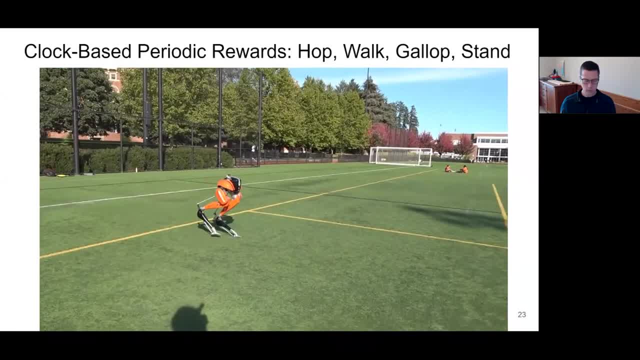 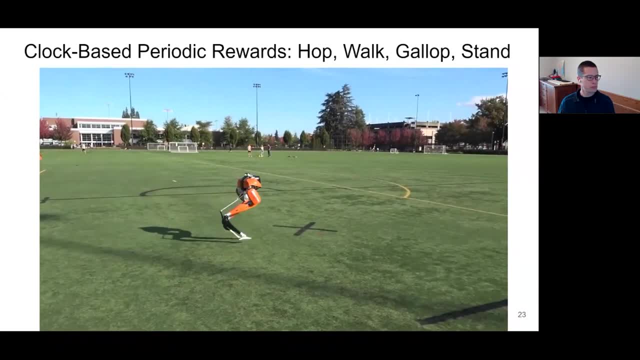 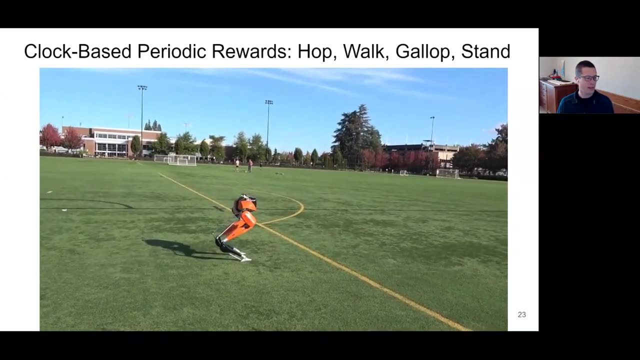 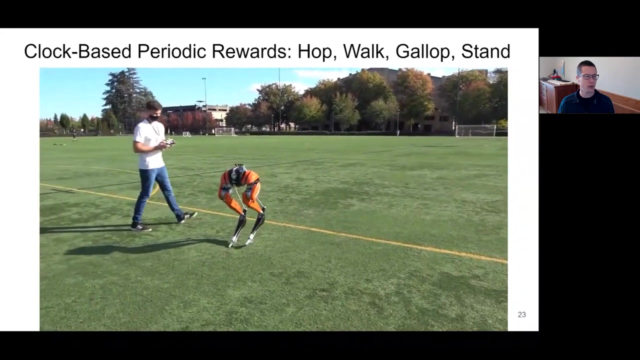 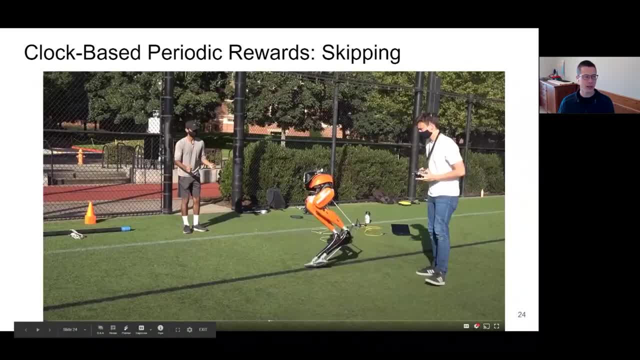 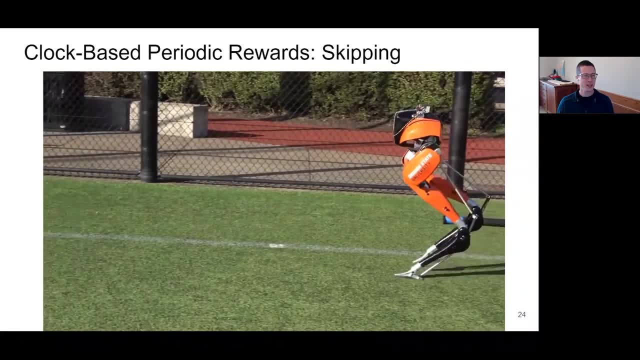 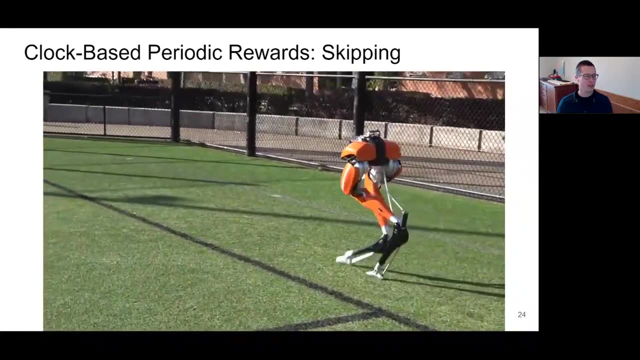 And this one is pretty cool. There's no good reason to skip, but we can. Any last thoughts? All right, change our clock cycle a little bit and make the robot look very happy. Nice sunny day outside. Off we go. We need to get a red hood for the robot in a basket. 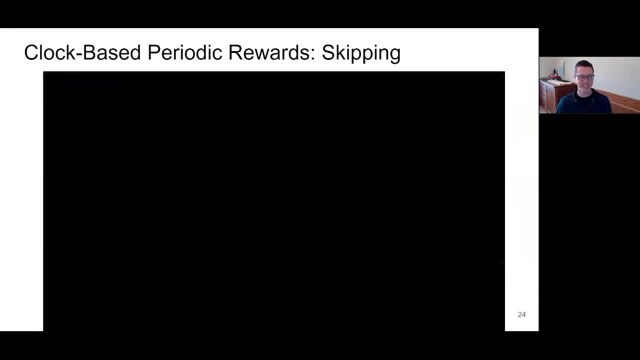 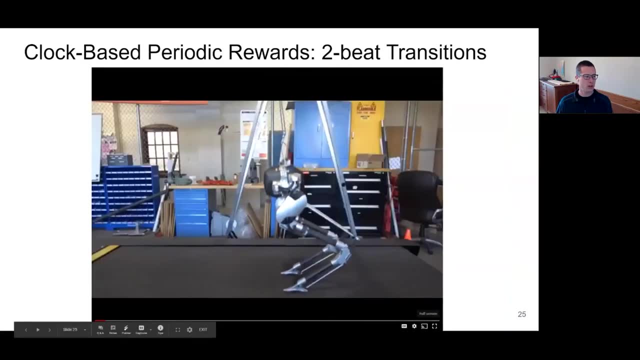 Oh, okay, I didn't cut out the fall, So when we're doing the clock cycles we can do a couple different options. You know here's a transition for the two beats, So really we can only do walking or hopping when we have. 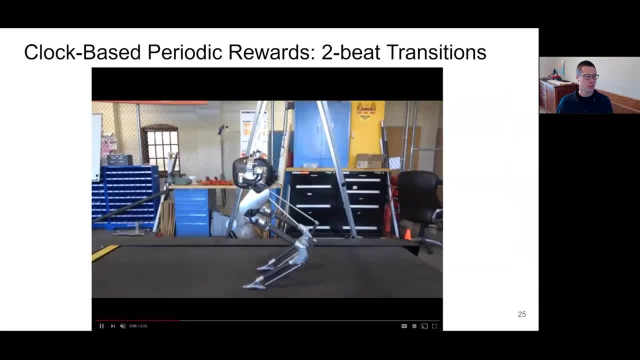 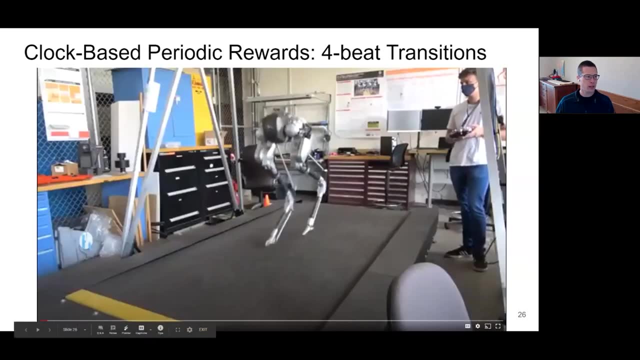 just the two beats for the gate transitions, But we can do the transitions between them pretty smoothly. And then if we increase the number of beats to a kind of a four beat transition, we can include a couple of other gates, like the skipping behavior and a gallop behavior, and transition between all of those. 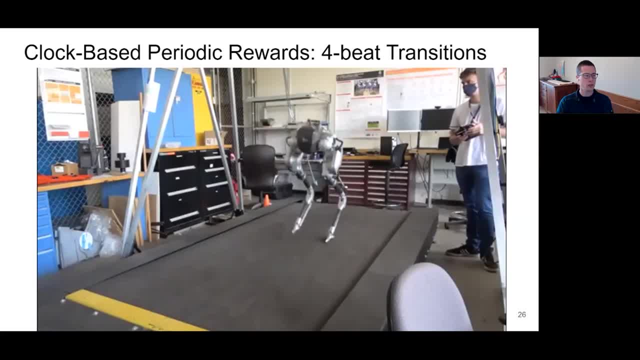 So this, by the way, is not task space control. This controller is learning all of the coordination between the joints. It takes quite a long time to train in order to do that. I'm sure we can do better if we split things up a bit, but getting some decent results this way too. 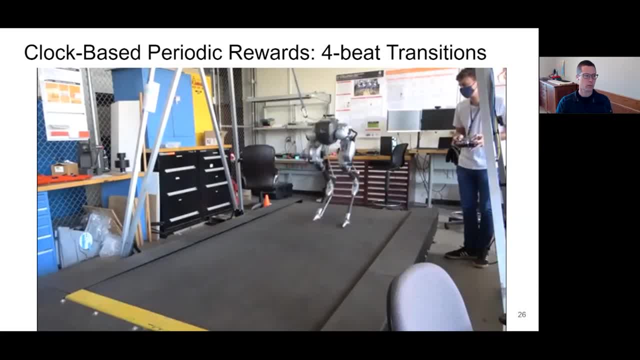 I was curious about this before. actually, Do you have like a one sentence? what is the class of algorithms you're using to do the training? It's a good question. The focus of this research is not on that. We're using old, classic. 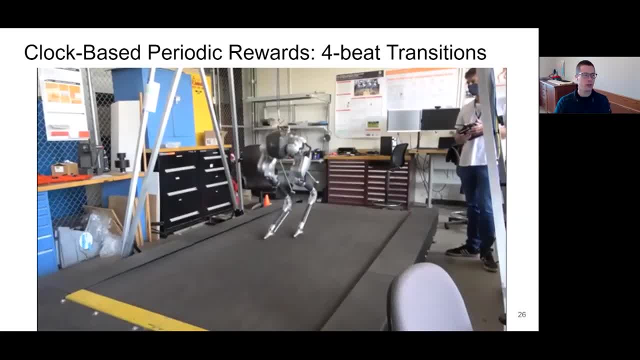 decade old kinds of algorithms. There's not a lot of innovation on exactly what algorithms we're using for machine learning. The innovation is entirely how do we structure the problem and how do we engineer it. I know I think this one was with recurring neural networks. 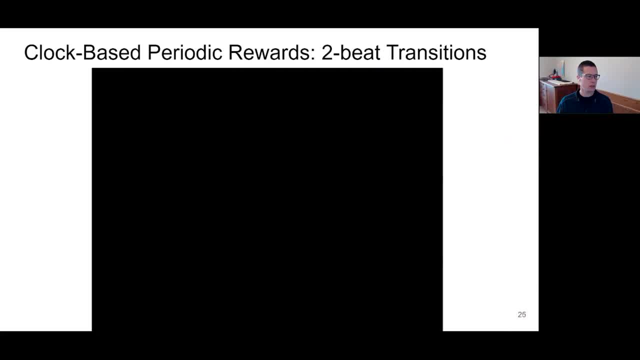 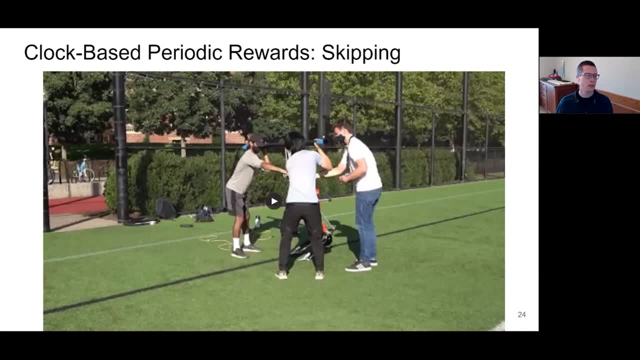 for some of these behaviors and for the skipping behavior. But there's also just feed forward networks that have no internal memory whatsoever. It seems like we're able to be secure in that. We're able to be secure in that. We're able to be secure in that. 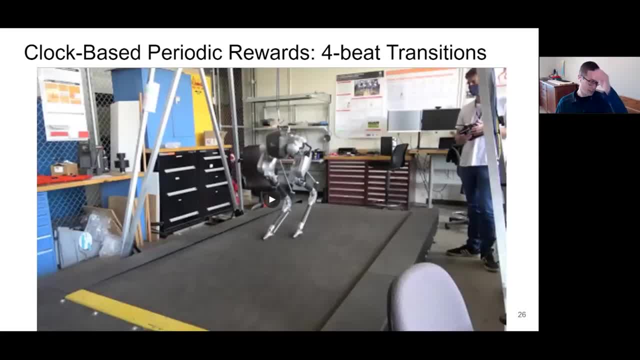 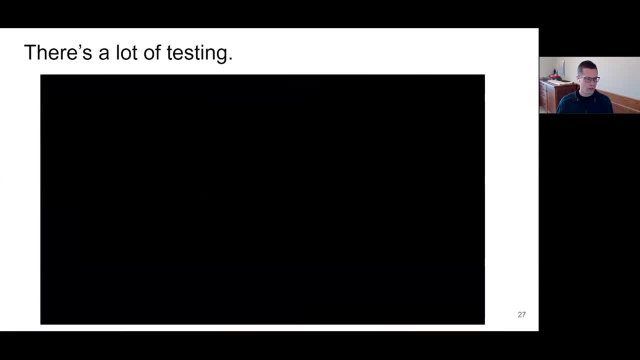 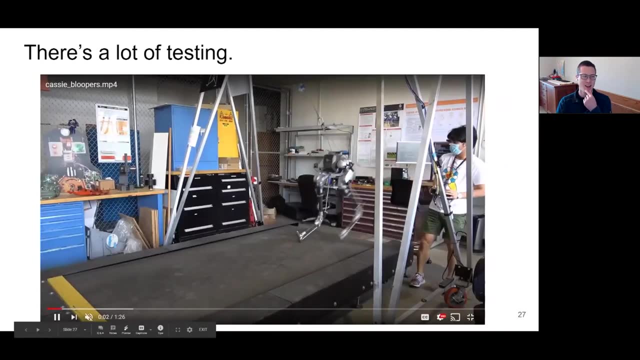 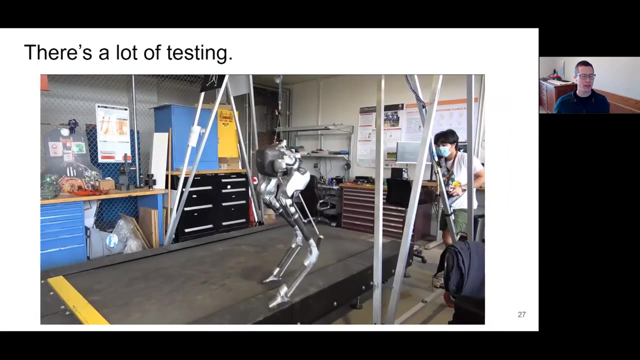 We're able to be successful with using a number of different approaches. Maybe that's less critical than setting up the structure of the problem. I'm getting close to wrapping up here. I want to point out there's an awful lot of testing, awful lot of falls Man. a lot of these have nothing to do with the learning policy A lot. 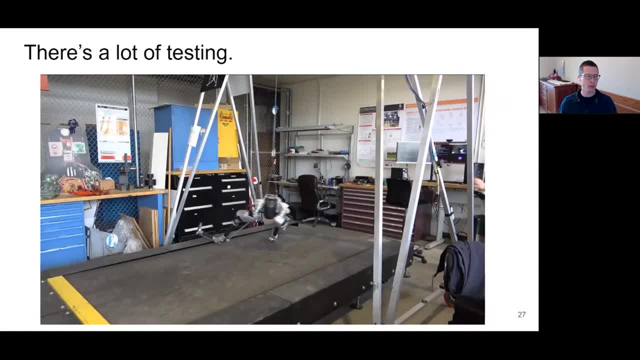 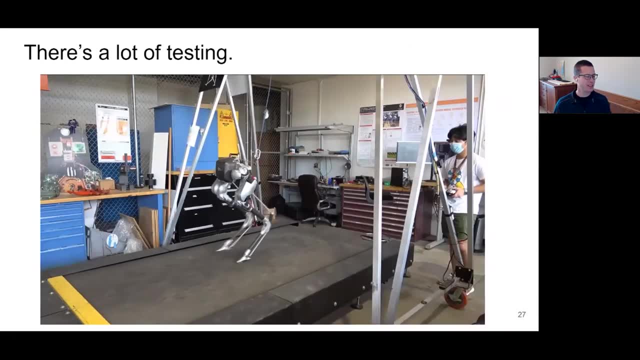 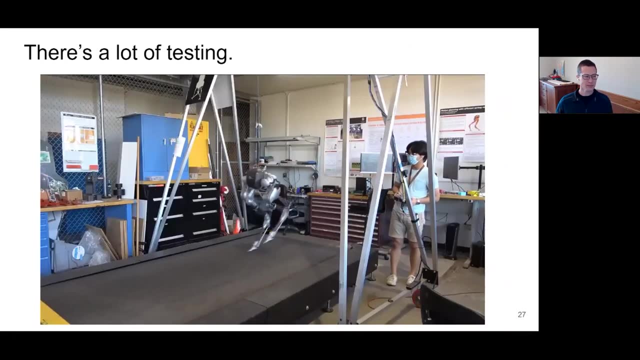 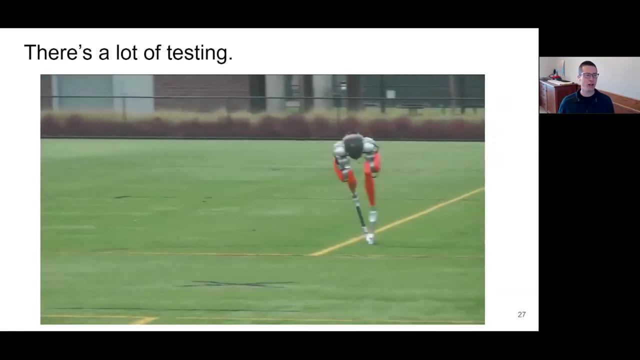 of these have to do with the state estimator was having problems or a part broke, or, in this case, whoever was controlling the speed on the treadmill wasn't on top of things, There's a mechanical failure. I love that one because it accelerated. It's basically getting a big shove. 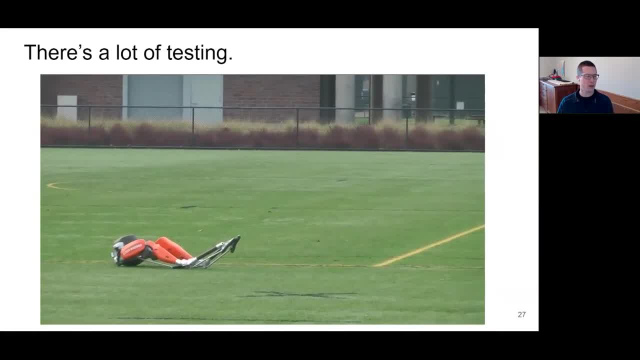 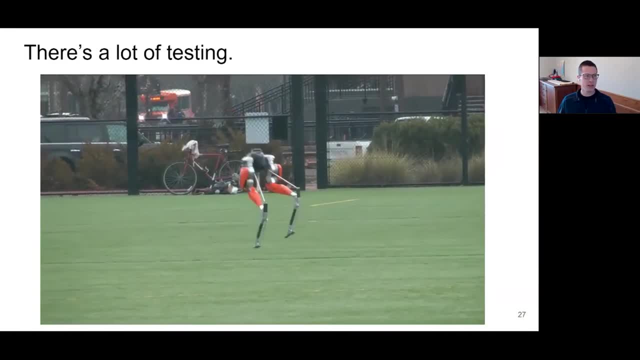 if the treadmill stops- and it didn't fall, It kept running forward. One of the problems we were having this day filming was actually data logging. Every now and then it would just pause the control outputs and the torque commands for a quarter of a second. 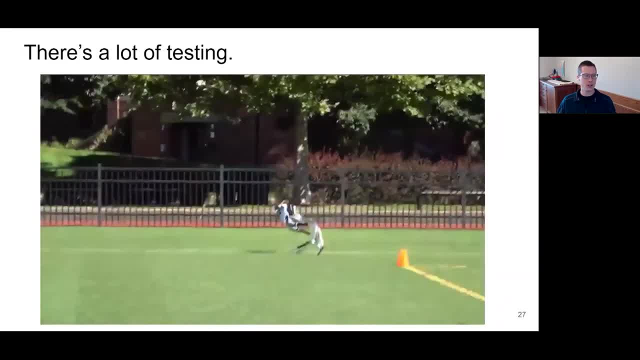 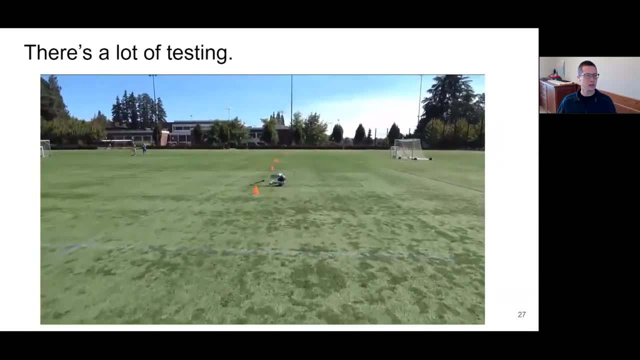 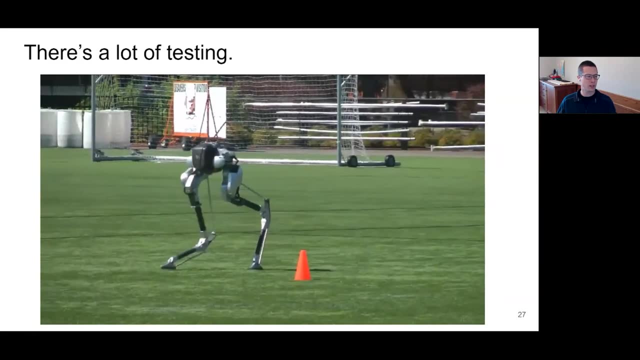 while it was trying to save a bunch of logging data That caused a bunch of these falls. You can see that leg just pause in the air. Having some hardware that's reasonably tough, that's pretty important. Having the support at Agility Robotics that's able to fix things. 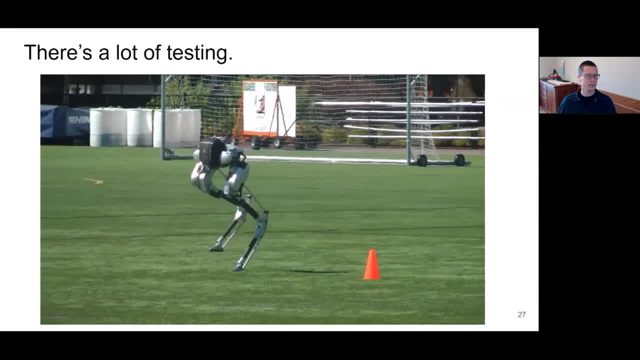 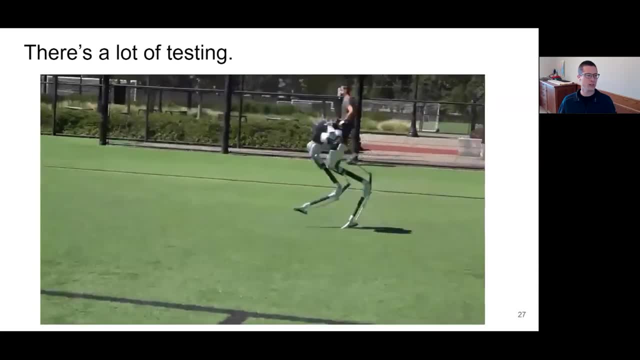 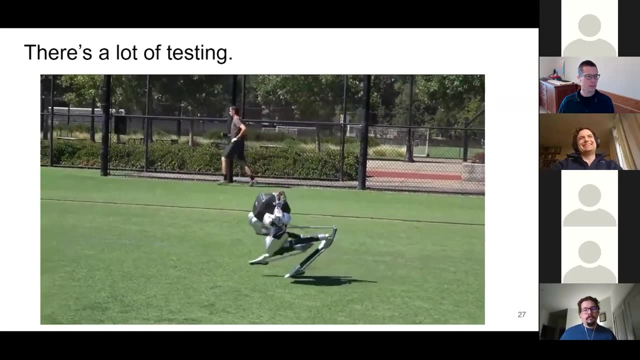 that's been useful There. That leg just paused and just didn't come down. The controller was telling it to, but the log files were being written. All right, I'll finish there. Thanks for listening. I'm excited to answer some questions now. 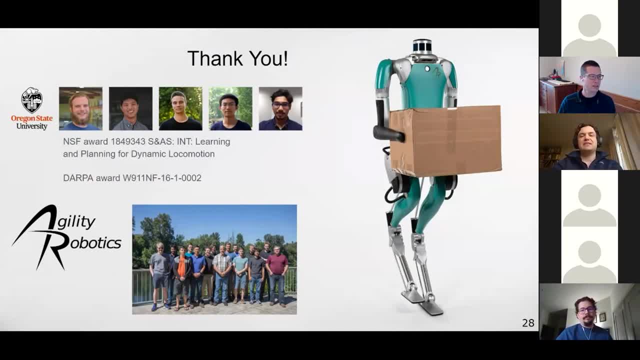 Okay, That's fantastic. Thank you so much, Jonathan. That was a spectacular gallery and constellation of ideas and just awesome, awesome results. Um, there was uh. I want to go to uh what I think will be probably a quick question and also just give you the. 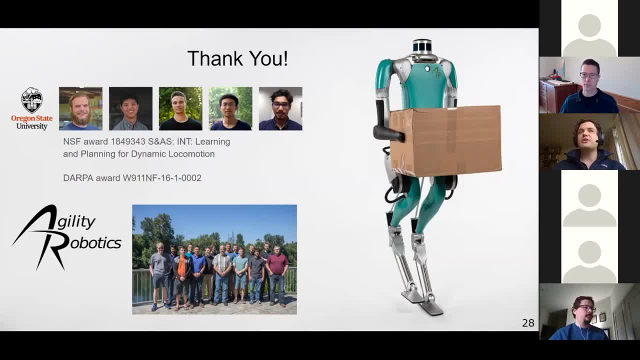 opportunity to, to do a plug. Um, there was a question that kind of halfway through: when can I buy one of these? So, like more generally, like what's what is available from Agility, You know what? what do you want to say about that to the people? 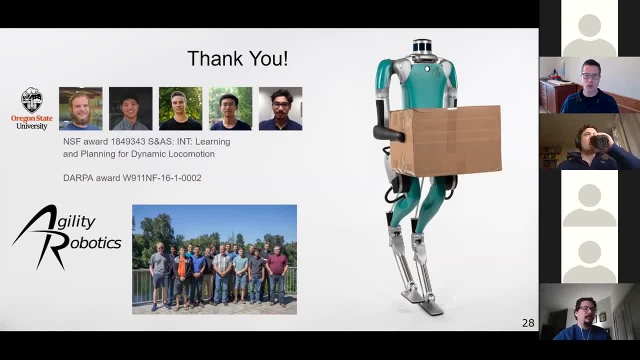 Sure, So we uh, we sold Cassie robots, uh, to some of the top universities in the world And, um, we are done selling Cassie robots Now we've sold about 11 of those. So when we started the company, we were about three people is when we sold our first Cassie robot. 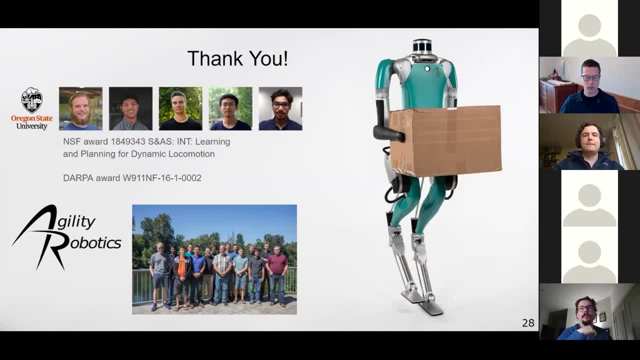 Um, and built the company on a kind of customer centric, building products and supporting them. um, making sure our culture, uh, was behind that Um. and now we're selling these digit robots which, frankly, are a lot more capable than Cassie. They have the arms and the upper torso and the 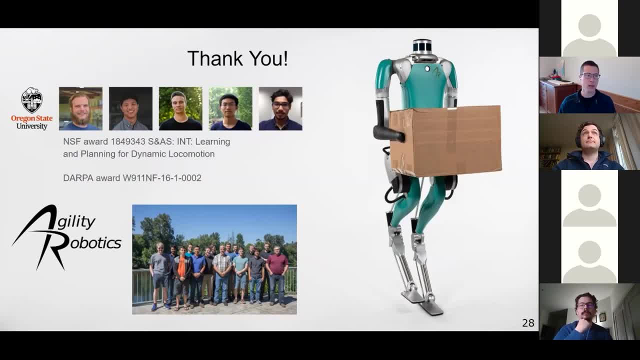 sensors and everything, And we're selling them for the same price that we sold the Cassie robots. We're selling these at $250,000 a piece. Um, and you can buy them now. We're selling. we are selling to the. 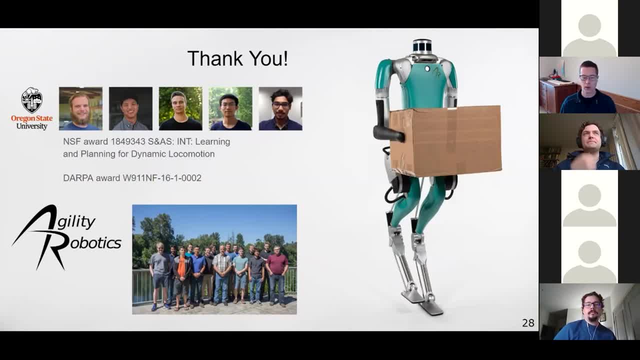 the academic market. Really, our focus is working with um corporate customers. Uh, we're aiming for the logistics market. We have these robots carrying packages around and there's a ton of backroom kind of work for carrying packages forward to the customer counter doing package. 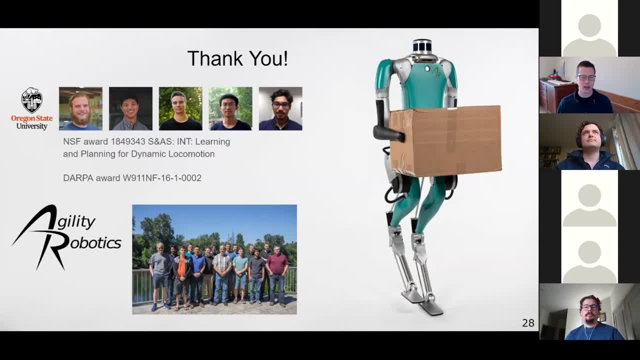 sorting, uh, stacking totes, a lot of the kind of classic three D's of robotics- dull, dirty, dangerous kind of work that still exists in a human environment. They haven't put in purpose built customized automation for it yet, And uh. 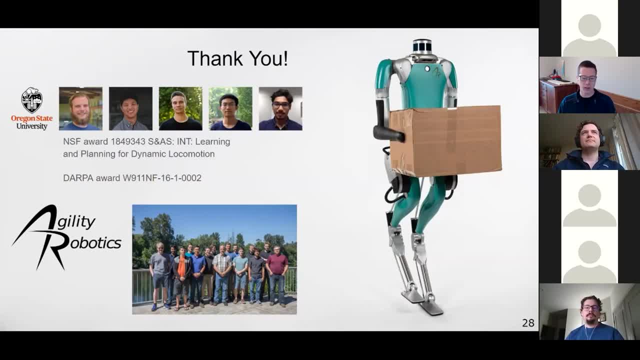 so digit is kind of perfect for sifting into a lot of those kinds of very robotic jobs that haven't yet been automated. Awesome, Uh, cool. So maybe, perhaps not, I don't, I don't know. Um the I don't personally know the person that asked the question, maybe out of reach for the private. 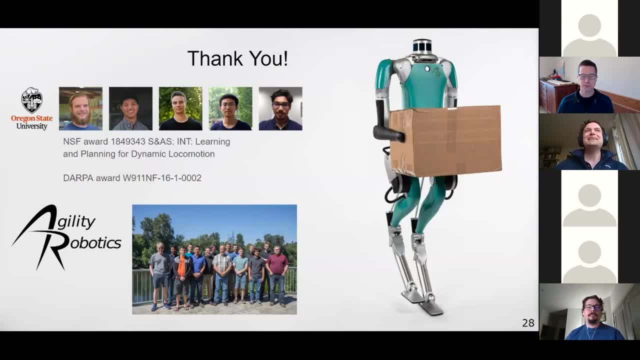 consumer at the moment, but, uh, but the research or or, uh, industrial customers definitely there. That's awesome, Um. and then there was an earlier question that I elected to kind of defer, um, that Joey wrote out and Joey can feel free to answer that Um, and I think that's a great question. 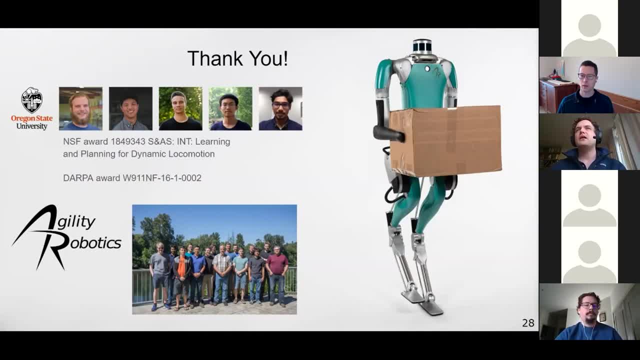 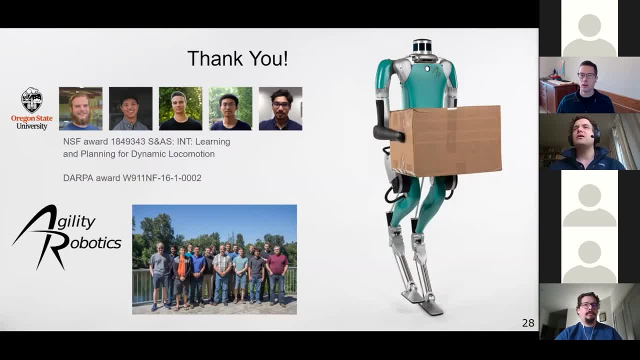 how well I can capture um the question. So, uh, I think the, if I understand the question, I think it's more directed at um, how does the class of behaviors you want a robot to perform? What does that tell you about the design of the robot? Oh, that's a great question, Um. 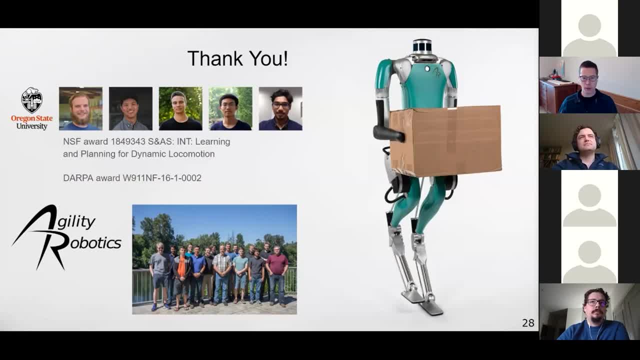 you know, we've been studying like locomotion for for decades and building on a whole community's worth of research in biomechanics and in robots, And just I think. a point I want to be clear about is: I feel that we are discovering 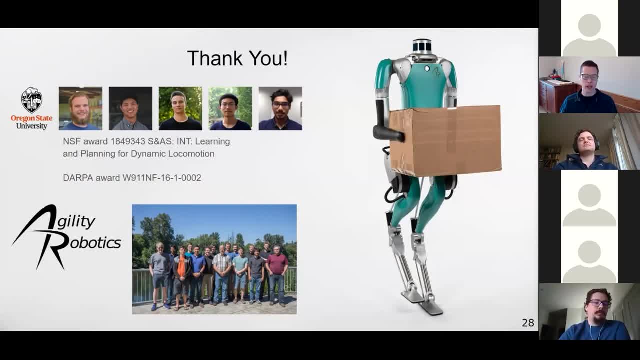 this dynamical phenomenon. Uh, and that's different from saying I'm going to design this cool widget- Um, Lego locomotion is not just um, what your imagination says, it is Uh. it is a special corner of dynamics that you need to be able to utilize. 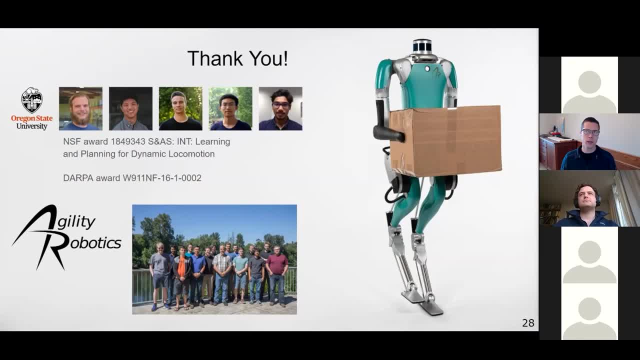 So knowing what we know is an input into the mechanical design of the actuator design, into the controller design, into everything about the machine. And you know we have, of course we have used no learning, machine learning in any sort of the mechanical design. I imagine someday that could. 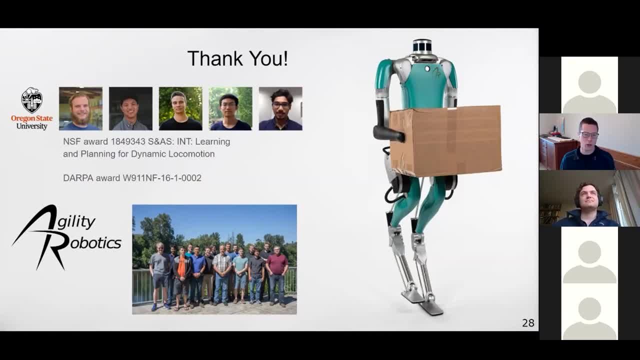 be a part of it. How can we optimize something about the spring function in the uh end effector of the leg? That's going to optimize for some behavior. We're going to see what the dynamics are that we want, which dynamics are going to optimize for some behavior, And then we're going 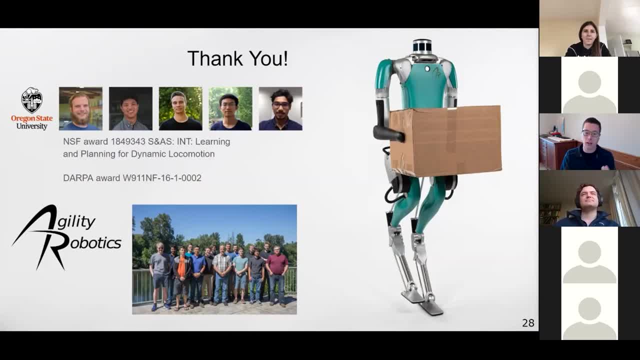 to see which dynamics ought to be on the side of the hardware and which dynamics, uh, ought to be on the side of the software. Um, to date, though, it's like we know we need compliance in certain directions, We know we need transparency in our actuators. Um, one of the reasons the leg on 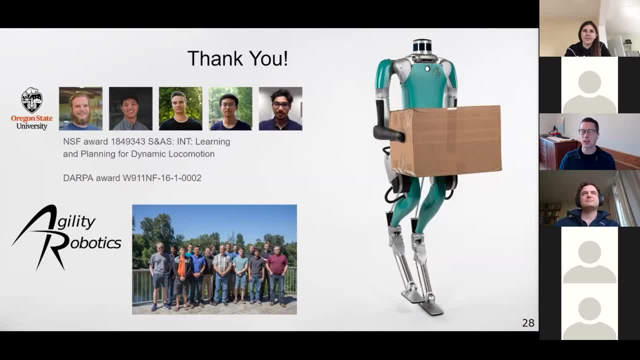 Cassie and uh digit is configured the way it is is antagonistic work. It's how much negative work does a motor do? And that's configuration dependent and task dependent. So Atrius, as an example, has to have the motors applied. 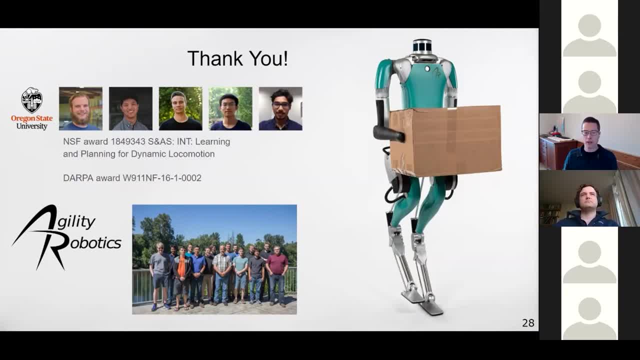 to the same torque at the same velocity. So what happens then is you've got opposite torques, but velocity is in the same direction. One motor is doing all negative work and one motor is doing all positive work, And so there's just this work loop where one motor is acting like a break all. 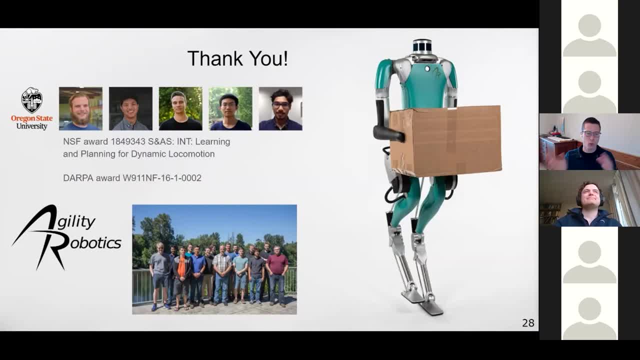 of the time, through all of the behaviors. And the other motor has to do all of the work on the world plus all of the work to overcome the breaking of of the negative work uh motor, And that's just a configuration choice. Uh, so the Cassie leg and 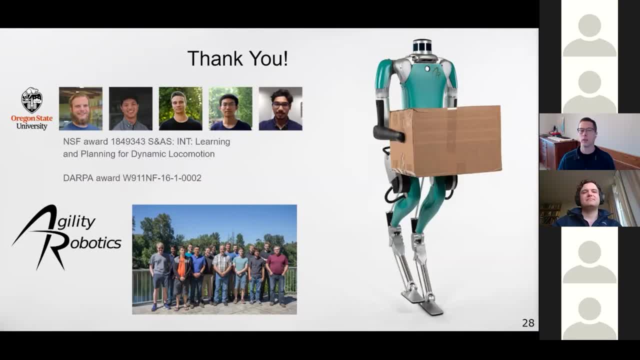 the digit leg avoids that negative work loop for the task of walking and running behaviors. Uh, so, walking and running forward or backward? Uh, it's just that you, we split up so that applying torques is one motor and applying velocities is another motor. to oversimplify, 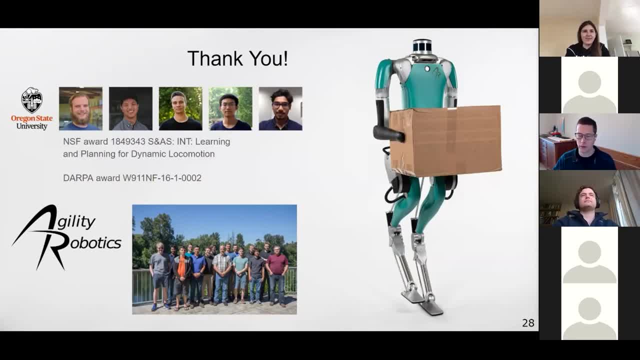 things a little bit so that you don't have them doing work against one another All the time. Uh, so there's just a lot about that kind of thing where you know your behavior, you know your task and you know the dynamics you're trying to engineer, And then it's a fairly 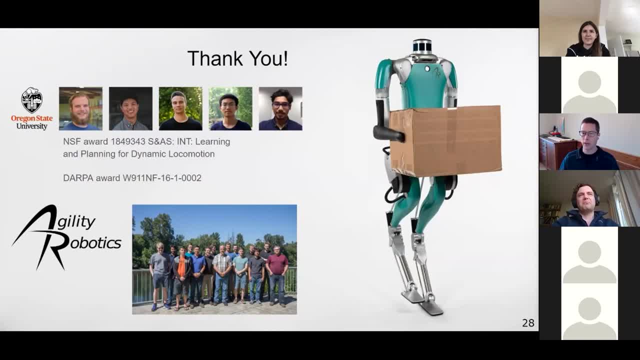 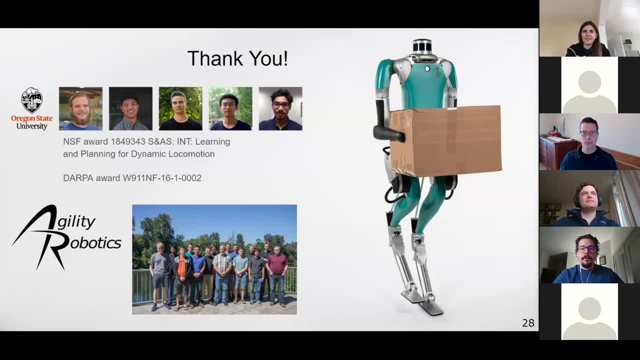 You discover a new one, or like that, there are many more important degrees of freedom. Um so is that information more important to informing the design of the robot or the design of the control Like? how do you distinguish between those two things? Well, um so you're trying to design. 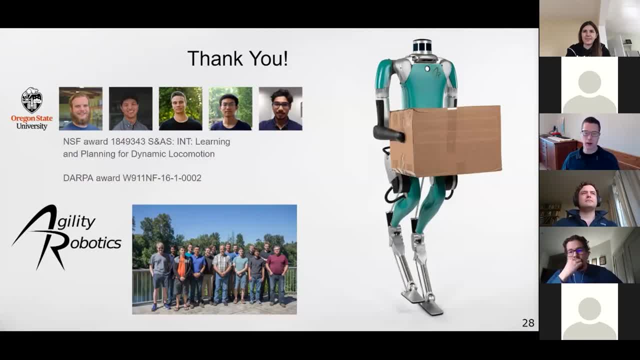 a set of dynamics and think of it like a control hierarchy in some sense. Like when you're riding a bicycle, the bicycle has its own dynamics, And if you take a bicycle and you just roll it in a parking lot and somebody- uh, you know, Andy arena and, um, Steve Collins did this, 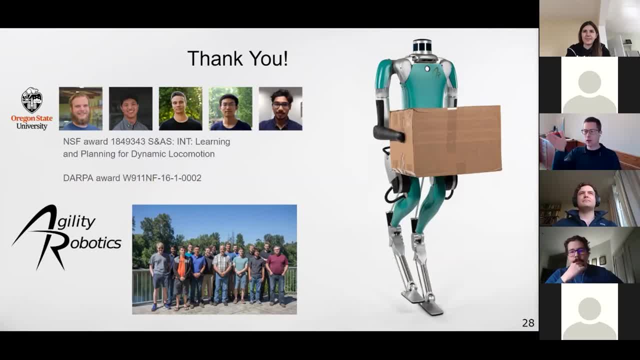 experiment. someone runs up and gives the bicycle a shove sideways. It tips over the steering wheel, tips in that direction, And then the contact patch of the wheels moves underneath the center of mass of the bicycle and it self-stabilizes. So if it's rolling forward, uh, you give it a sideways. 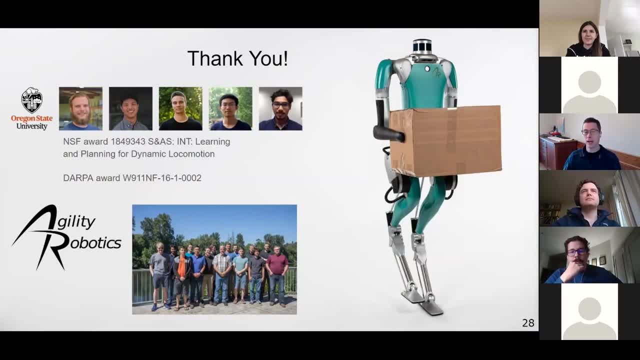 shop, it's self-stabilizes. And then you take a bicycle and you just roll it in a parking lot. And then you take a bicycle and you just roll it in a parking lot and it self-stabilizes, And you are relying on that self-stability of the bicycle in order to ride it. Um, now you can make an. 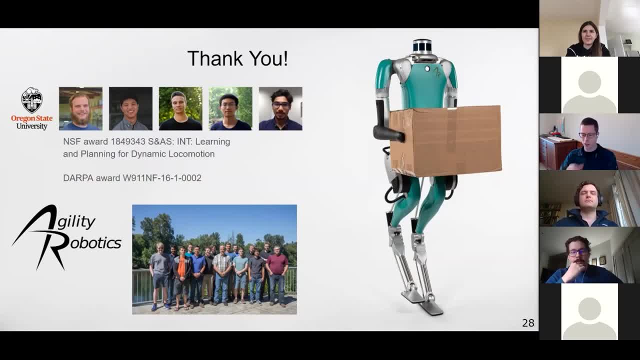 unrideable bicycle by changing the pitch of the of the steering columns. Uh, and then you can either balance on it or steer, but you can't do both. Uh, I think there's some analogies in aircraft. Uh, some aircraft with a big dihedral wing gives you a lot of stability. Uh, in that. 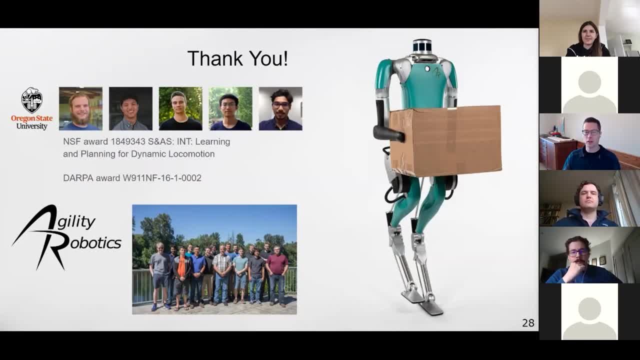 case, it's a trade-off though, because, uh, fighter jets and things that need a lot of um, you know, uh, um agility have the inverted wings, So they're really unstable and they always have to stay. You have to really be on top of it in the controls in order to stay stable, So I don't. 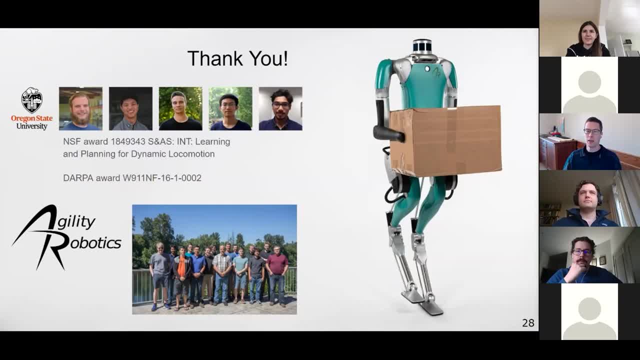 really know how to answer your question. It is a big, complicated engineering problem, And it's an engineering choice to decide what is the set of dynamics that your hardware has that you then are constrained to. Now, you must work with the dynamics of your hardware, Um, and, and then your 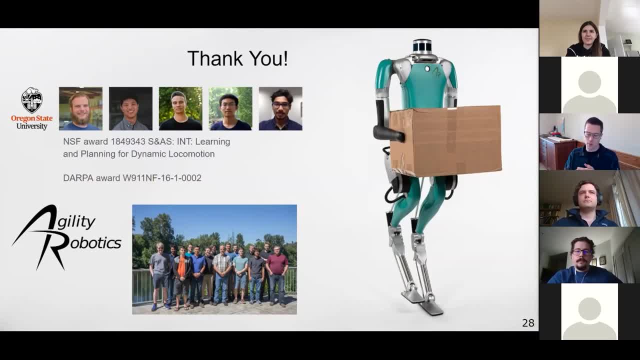 control input is able to work with that. So I kind of imagine it like if you're thinking of the, you know, five or six layers of a control hierarchy which are all divided by control rate but also information content. at some level you have a dynamical system that really captures. 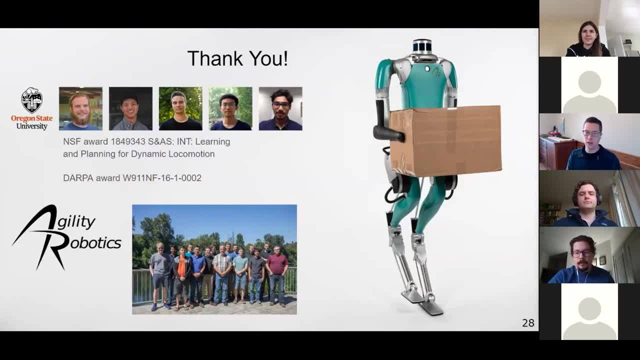 something like the spring mass system, but in 3d. uh, but also handling contacts and impacts, and also including your actuator dynamics and so on, You create a set of dynamics. You've got a whole range of behaviors that you can now. 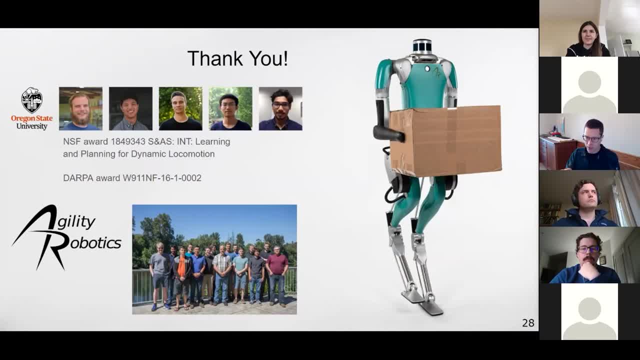 Maybe five different degrees of freedom as an action space for inputs into this, to have your attractor land in different cycles or different behaviors. Uh, and I think there's going to be a lot of choices about how you design your hardware so that your behavior is above or below. you know. 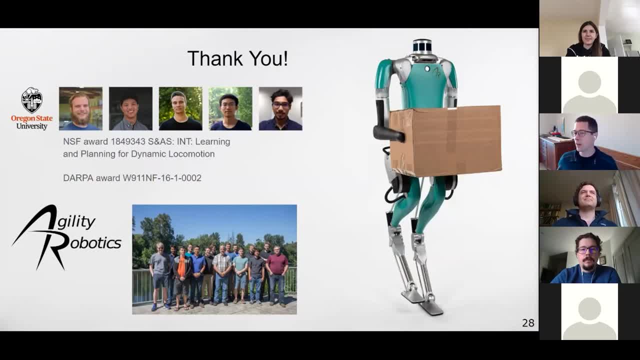 that line. Um, I don't know, not a very satisfying answer, cause I don't know the answer. Uh, and I think there's there's still a lot to discover. Thank you very much, Cool, Um, we may have time. 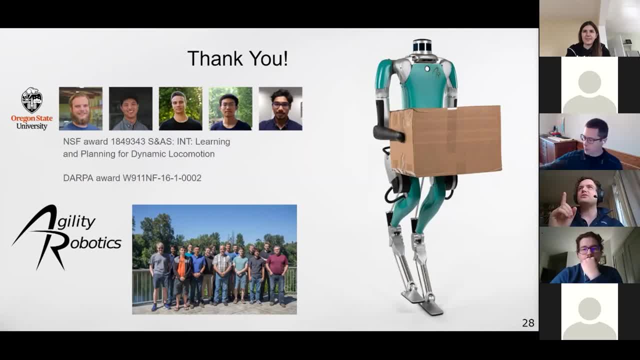 for just one more question, Cause I know Jonathan has a meeting Um, I'm going to ask you a question at the meeting um at 1130, and I saw Kat Steele's hand up, So I'd like to give her an opportunity. 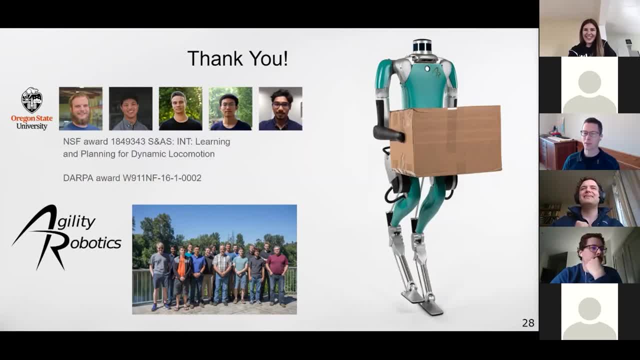 Megan's question first. It follows on nicely. Megan asked in the chat: uh, could the robot adapt to alter dynamics? For example, if the it's framed, its ankle- I mean, if you're aware of it, our robot typically isn't So when- when the ankle loses its actuator direction? um, it, it, it. 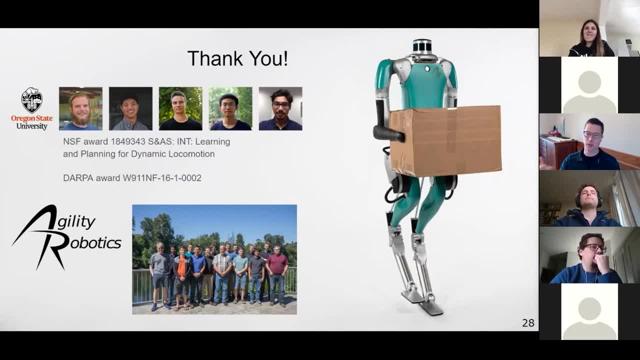 stumbles in a weird way. It treats it like a disturbance every single time and never plans for it. Now I will say that uh, with digit, were a lot more able to identify Failures in encoders and sensors or actuators and things like that. And then, yes, the optimizer very quickly, uh adapts to it. So, for example, 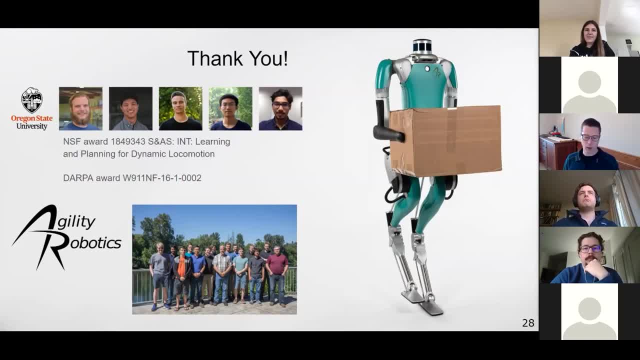 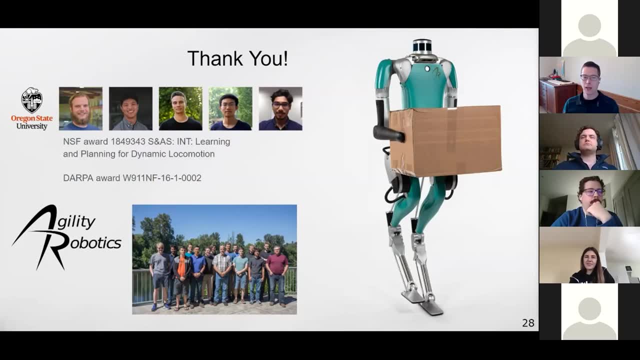 if you're walking along and the arms are swinging because one foot is on the ground, applying forces the ground, the other leg needs to swing forward to its next position, That's applying torques to your body. Uh, what are the best inputs in order to temporarily mitigate those? It's it's swinging. 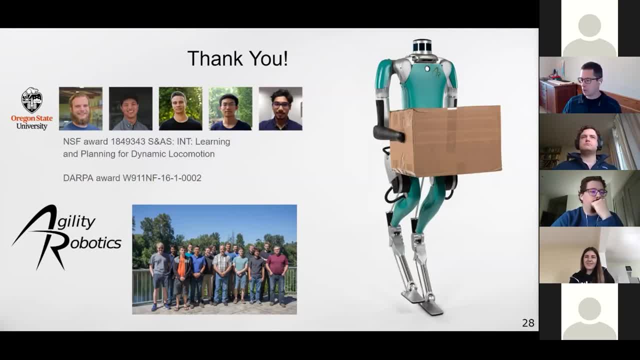 the arms at inertia. Anyway, let's get into this. So, uh, before we uh talk about the dynamics, uh and uh, if you are carrying a box and the robot knows the mass, it works right into the uh optimization to swing that box an appropriate amount. or if you actually remove one of the arms, 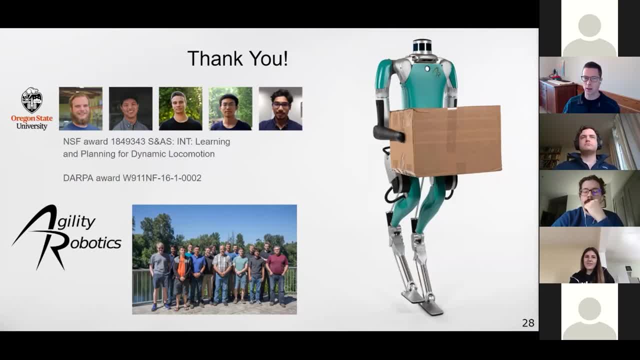 uh, it also the optimizer very quickly. uh is able to just compensate for that. the other arm swings a lot more aggressively and and more across the chest a little bit. so in some ways, yeah, it definitely does adapt to altered dynamics, as long as it's aware of what they are, something like. 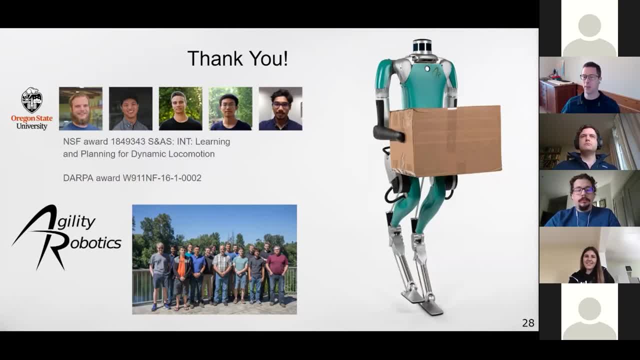 removing an arm. it knows what the arm's dynamics are and is able to adapt. very cool. that's why i love some of your failure videos. um, it looks like there's enough time, so i'll ask my question then too, which is also related to the legs and the feet. so can you talk a little bit more about the design? 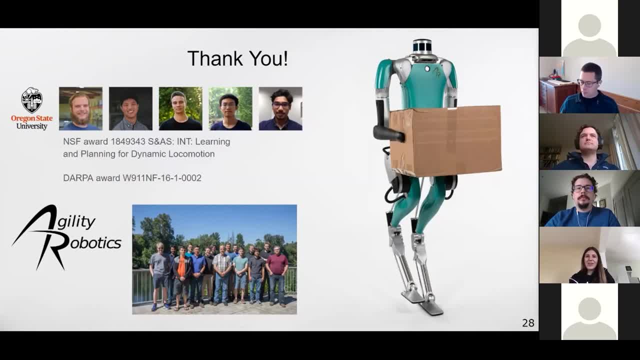 choices around the feet. you know, you mentioned a little bit how you know, especially cassie, they're so small and rigid. it looks like digit is a little bit bigger, but yeah, i'd love to hear more about that process. good question. so you know, early on we built a spring mass robot, atrius, and it had no feet whatsoever. it had a rubber nub. 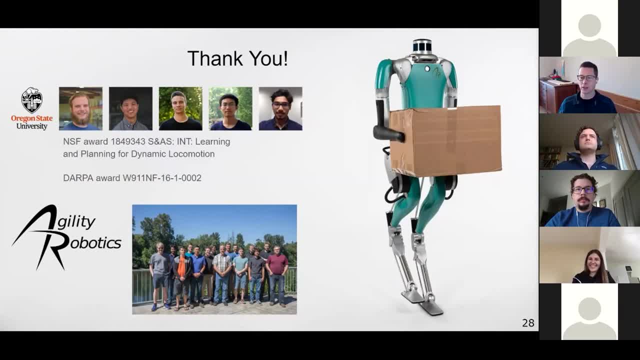 on the end of each foot, because you don't need feet in order to walk or run. it's just not necessary. but one of the biggest failures is the robot rotating sideways, and then its velocity and its orientation are no longer aligned. and so it it's. it got up to speed, running forward, but now. 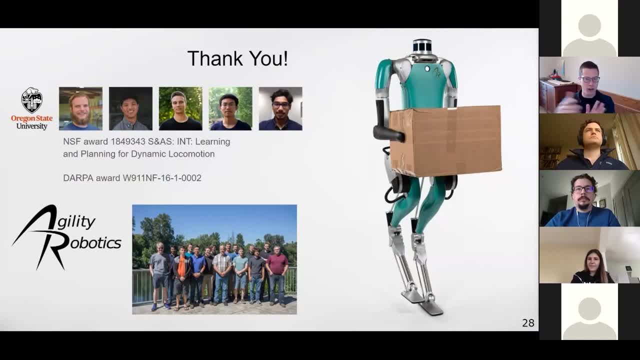 that that velocity is pointing sideways relative to the robot and it's trying to sidestep frantically to keep up with that speed that it had and it falls right over. so we had to add little kind of passive feet with a little bit of foam just to try and keep the 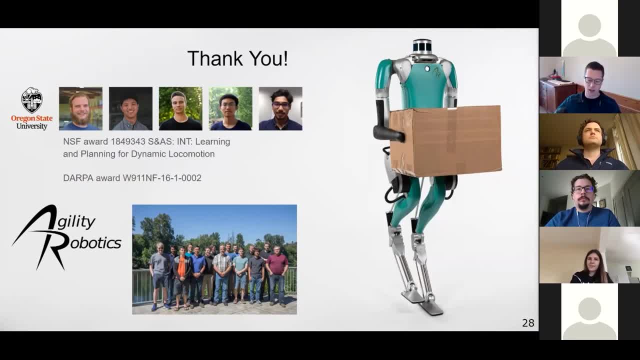 feet roughly flat when it was in the air, so that when it placed the foot on the ground the foot would just slap down on the ground. but prevent the robot from torquing too much and just to provide a little bit of yaw control now with cassie, and that's one reason atrius could never stand. 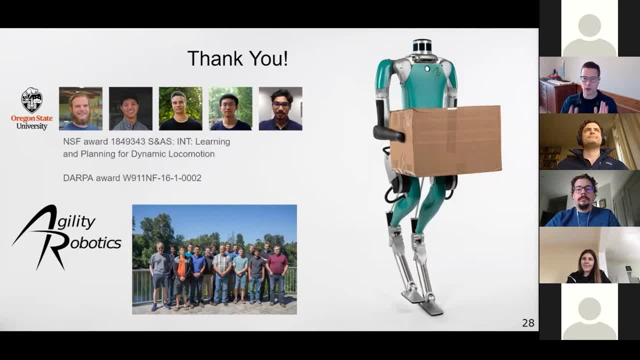 because it had no ankles. now cassie had ankles, but only in the fore-aft direction, so it's like walking on an ice skate, perhaps, where you can stand if you've got both feet down, and you'll need to be able to keep the feet up where you want to lean them down, and it's a little bit more comfortable. 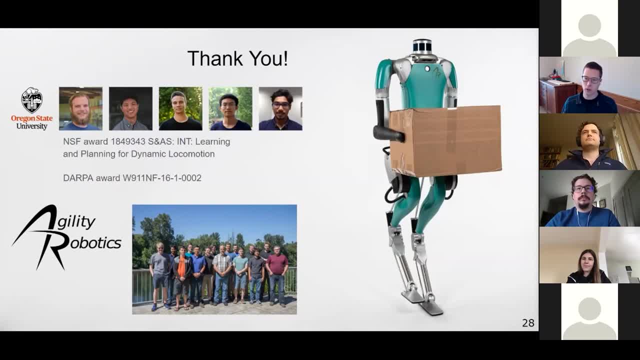 if you can stand, if you've got both feet down, so you don't have to use the legs with the legs up because they're low. so that's the reason why you won't have to try and bend and try and fix that- both feet down. But of course if you only have one foot down, you're falling to the right or left. 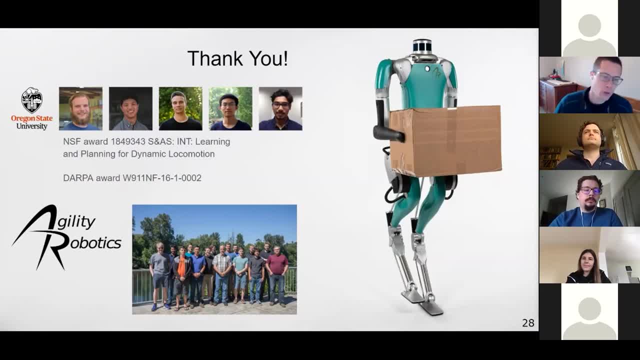 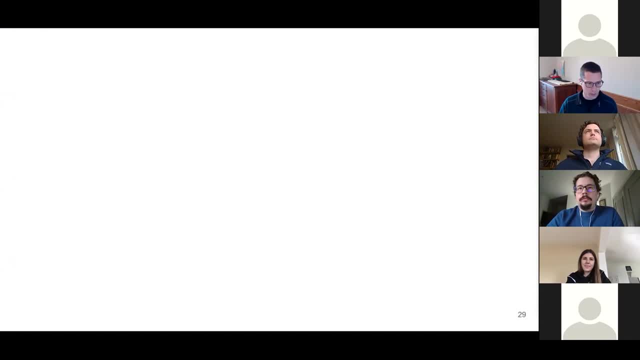 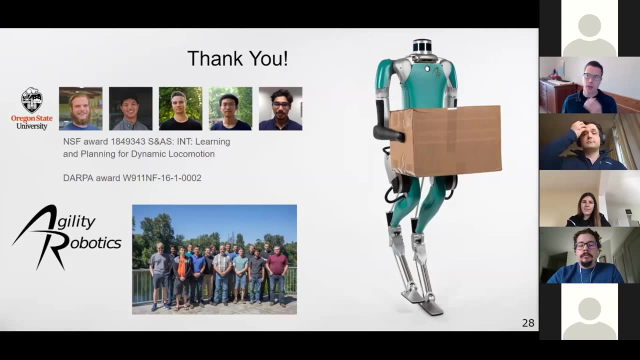 at all times. So one of the drawbacks to that actually was: you know, I might even have that video here. Oh, I don't. unfortunately, We were doing the testing with the early version of digit going up and down stairs And because you have no way of controlling the center of pressure under 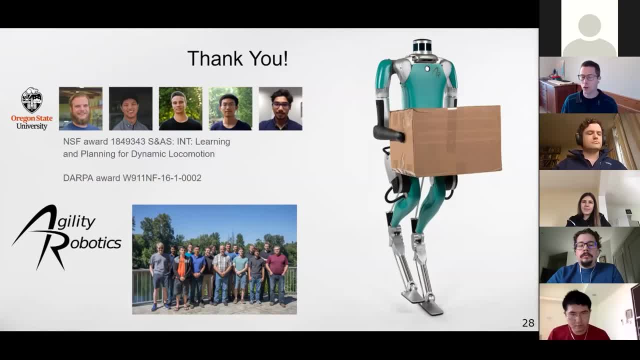 the foot even a little bit during stance, you are always falling and you're going to need to get your next foot down pretty quickly, And the longer you take to get your foot down, the farther away you're going to have to put it in order to make a correction. So going up and down stairs. 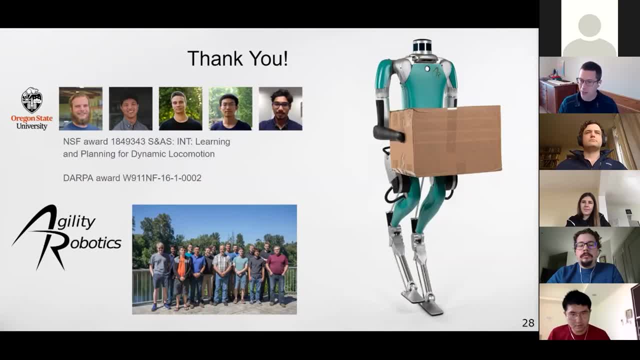 you have to go fast. You can't go up and down stairs slowly because you have to place your foot really quickly. So adding the second degree of freedom in the ankle is a kind of a pragmatic choice where we're kind of wrapping in some of the traditional humanoid zero moment control kinds of. 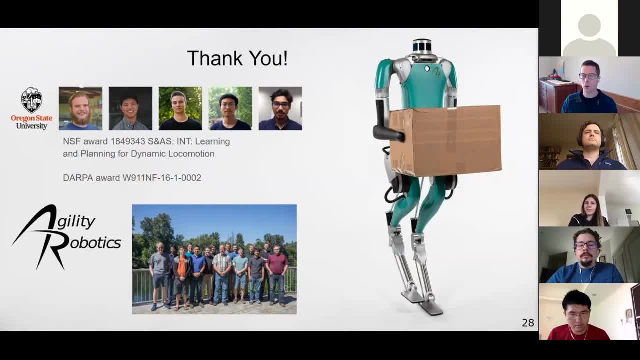 ideas here so that throughout all of stance you can apply some torque and just correct some of the small errors of where you place your foot placement. It's another control input that allows you to go slower up or down stairs. However, now the lower feet are getting. 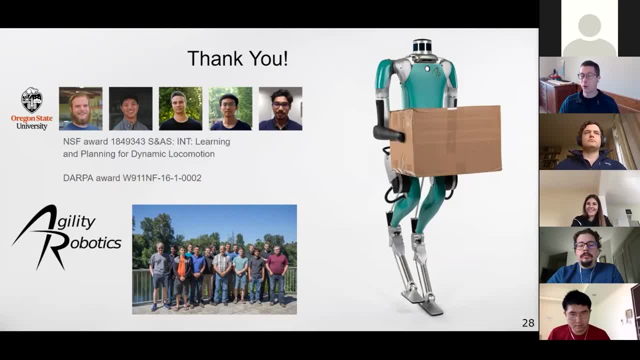 pretty heavy And you know, it starts to get pretty clumpy and we start to have to think about how are we going to deal with that inertia on that contact point. And so some of our research has been understanding that and figuring out how to handle that impact with the ground while still 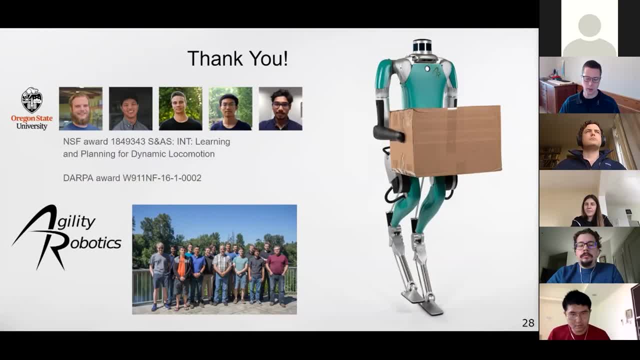 enabling the mass of that, that inertia that we're adding to the end effector. Certainly, human legs have a lot of mass compared to something like an ostrich, But our feet are pretty different from an ostrich as well. Also, ostriches can run 30 plus miles an hour, can do a marathon in, you know. 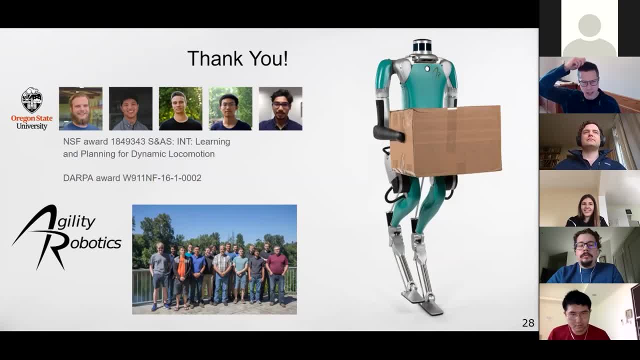 some ridiculously short amount of time. I want to say 40 minutes. I can't remember the exact number, but they're much better for long distance running over terrain than we are. Anyway, that's a bit of a story about the feet and the evolution of our feet, And they're going. 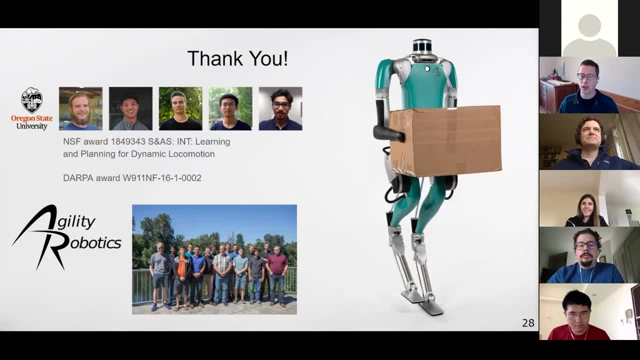 to keep evolving, because there's a lot of interesting dynamics that happen in the feet during contact with the ground and for adding energy into a gait or behavior, And it really influences what we may want to do with leg configuration in the future. I just like to try to ignore them myself.